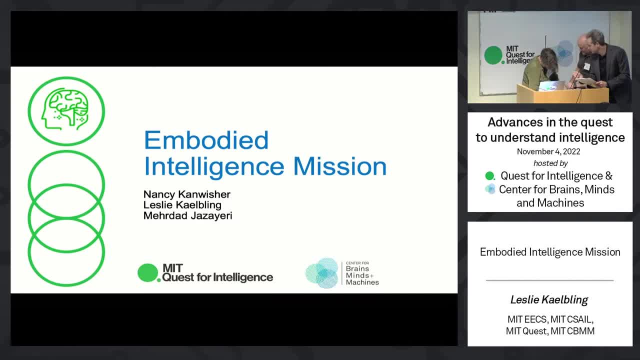 some domain of intelligence. You'll hear about several of them today. First, you're going to hear from a team of people- Leslie Cabling, Nancy Kanwisher and Murdad Jaziri- about the status of something we call the Embodied Intelligence Mission. So, Leslie, go All right. thanks very. 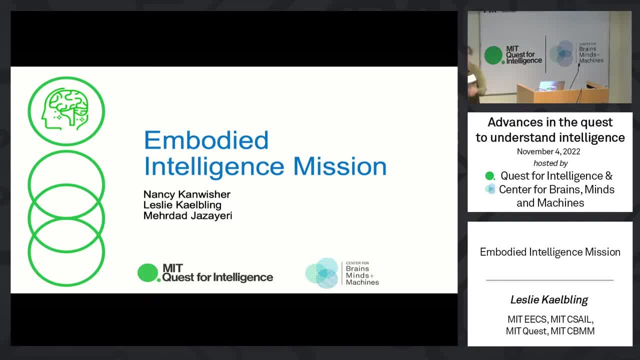 much So. I'm Leslie Cabling and I'm an engineer, so it's a little bit of a change of emphasis and focus. This is a talk that I'll be giving with my colleagues Nancy and Murdad, and we are going to 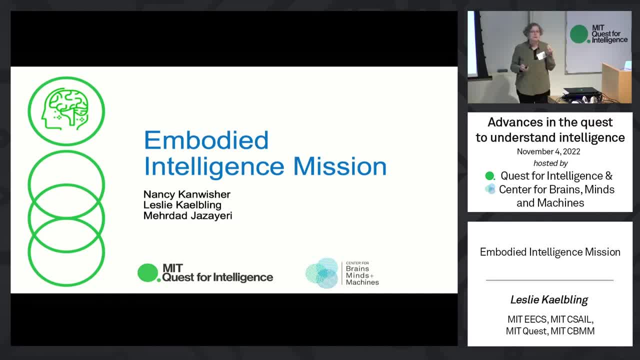 talk about one of the missions of the quest, and the mission is in embodied intelligence. So the fundamental question is: how is it that our bodies actually affect the way that we think about the world, and how do we make intelligent agents that demonstrate their intelligence? 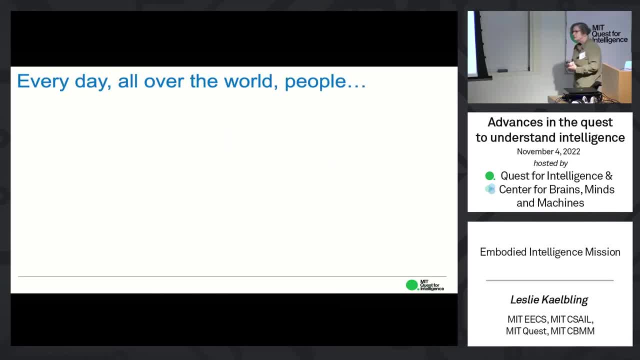 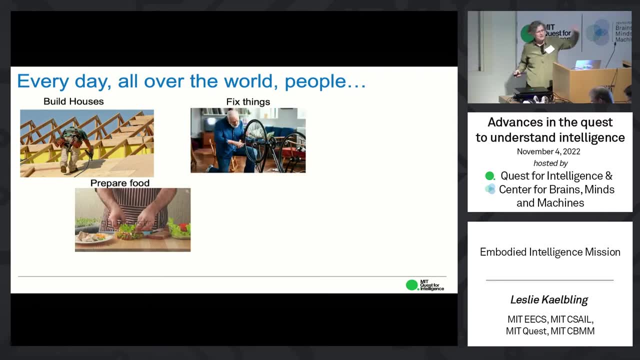 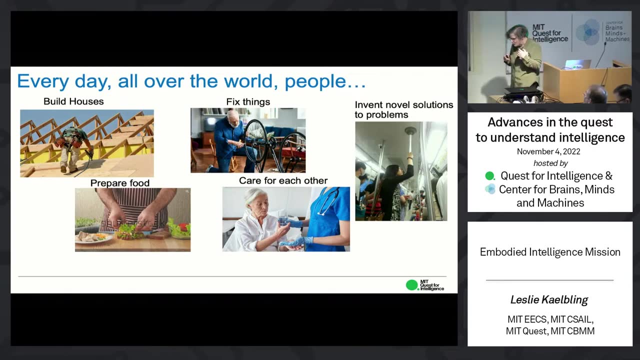 via their interaction with the world. So if you look at what people do, they do things with their bodies in their hands all the time. They build houses, they make food, they care for people, they solve problems in interesting new ways And, fundamentally, intelligence shows up in all of. 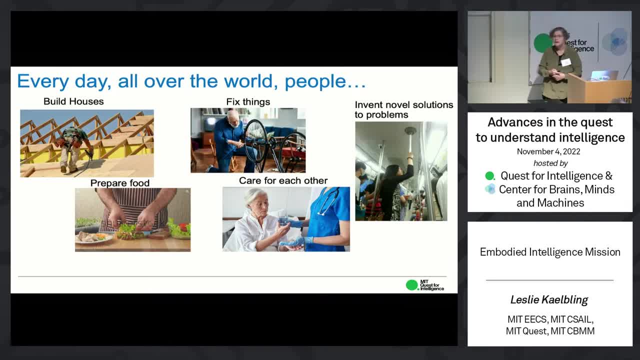 these interesting ways that people interact with the world around them. And so if we think about robots- so if I come from engineering, I come from robotics- I think about, well, how can I make robots that are able to do all of these things? And I think about, well, how can I make robots? 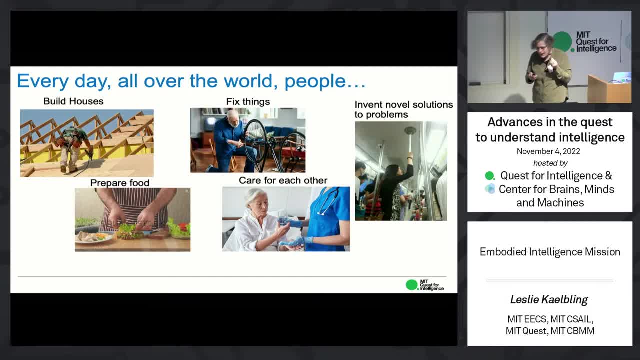 that are able to do all of these things, And I think about: well, how can I make robots that are able to intelligent, and what does it mean? how is it that the intelligence really helps a robot solve a problem? So when we think about robots, often we think about very stereotypical robots solving. 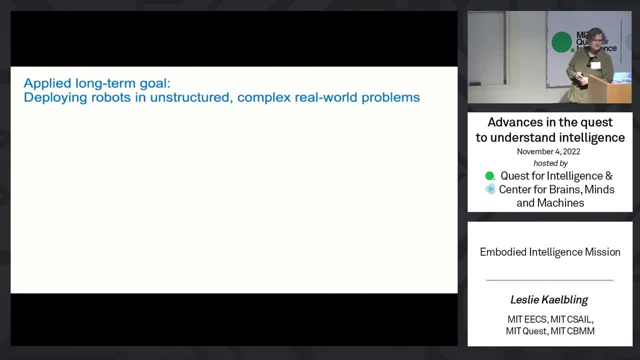 stereotypical problems, but our interest in this mission is in actually solving problems of the kind that humans solve. So how could you take a robot and put it in something like a disaster site and have it react appropriately to all the wild and crazy things that could happen? How could you? 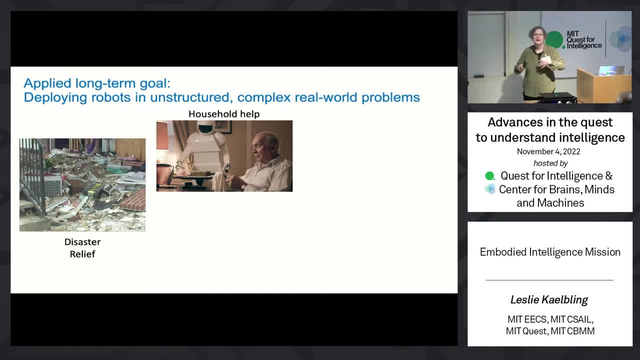 take a robot that could really solve a problem, and how could you take a robot that could really help a person in an open domain house with all kinds of new objects and problems to solve, to work on a construction site whereas we all know nothing goes exactly according to plan, or to work in a, say, a supply depot? that 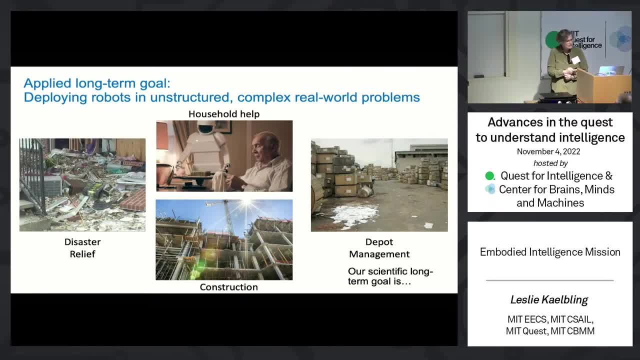 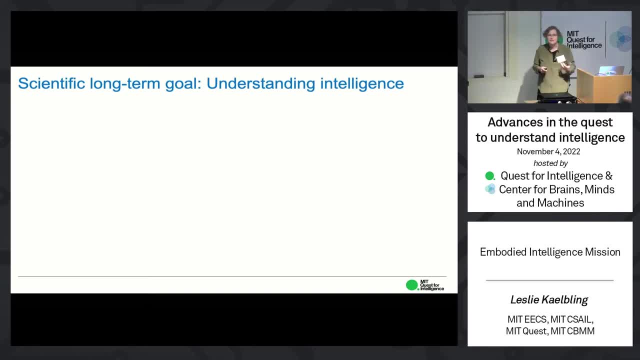 has again a great variety of things to do. so what do we have to do to make this happen? well, we have to build up from the engineering, but we also have to really fundamentally understand the nature of intelligence. and Josh just slightly stole my thunder here, but I'll take it back. I'll take it just right back and 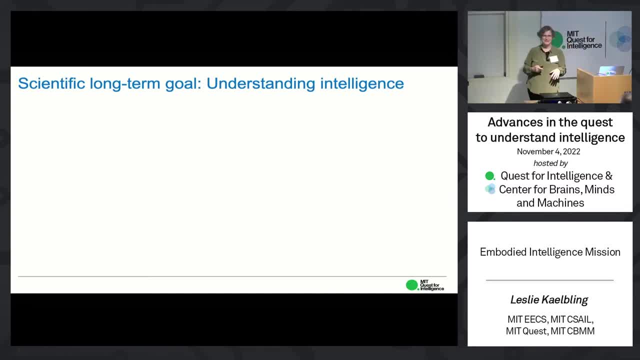 we'll say: well, okay, so how are we gonna think about building these intelligences? right then, what is the underlying science? and, of course, a brain in common science. for years, people have thought about this. right, they've developed models of neurons and neural circuits. they thought about how you could build. 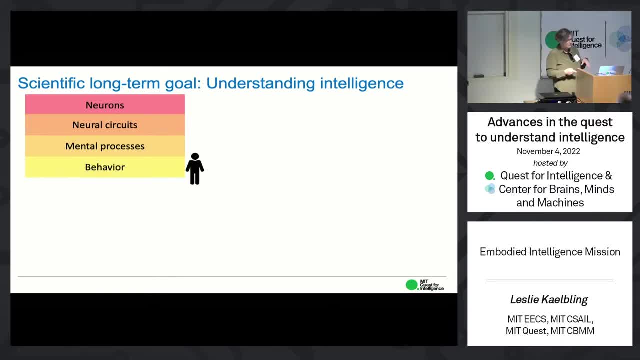 on those circuits by understanding the mental processes that run on top of them and how, ultimately, they give rise to behavior in humans and other animals, and how people who study neuroscience and cognitive science try to build theories of this kind of intelligent behavior. at the same time, on AI, we've been replicating or 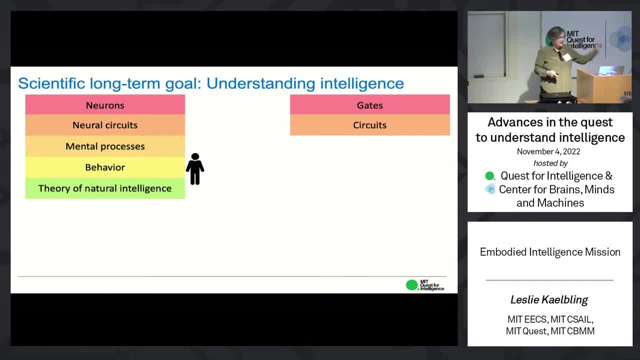 cross-pollinating, and so we've built system with gates and with circuits and thinking about how algorithms run on top of them and how that can generate behavior in robots, and AI theory is a thing. so that's. there are two kind of parallel processes. there's another process which is coming up from theory. 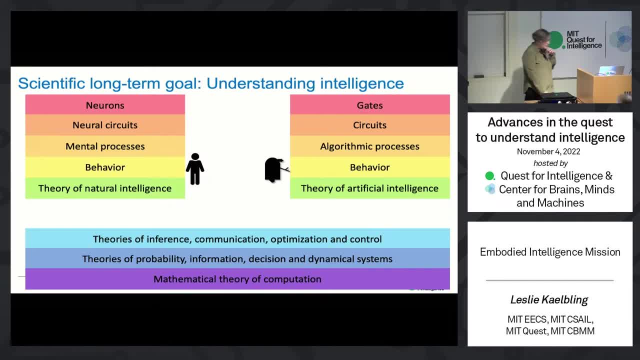 right. so there's math and theory of information and computation and so on, and what? what we're really after is a thing that's missing in this picture, and it's a thing that connects all these parts together strongly, and so I put my bet- we're putting our bet on this notion that there's a general idea of intelligence. 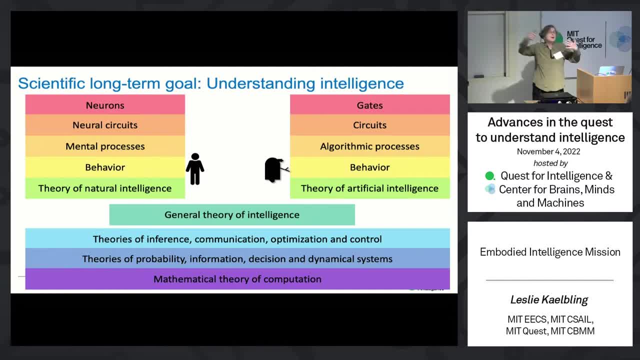 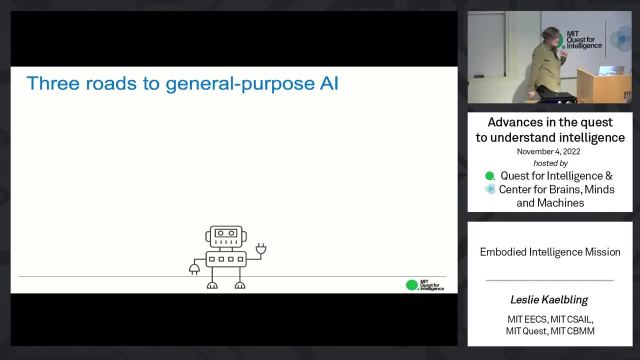 and one kind of intelligence is what you find in nature. there might be other versions of intelligence that you find in artificial systems, that- but by studying them collectively we can arrive at an understanding of intelligence as a particular kind of process that happens in many different contexts. so okay, so let's just take the robot. 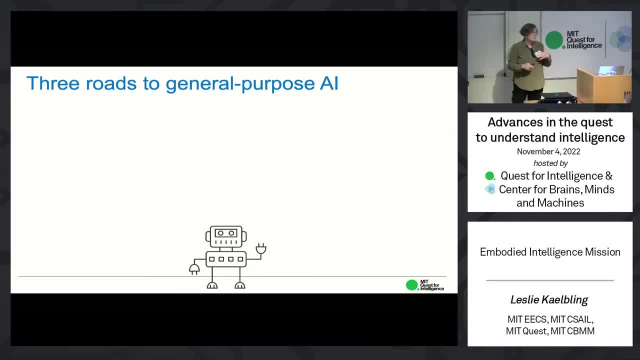 perspective for a minute and think about how are we going to make intelligent robots? and there's a bunch of different strategies. people are placing their bets differently. one category is reverse engineering: humans. it seems like if we could understand exactly how humans work, we could replicate them and we could. 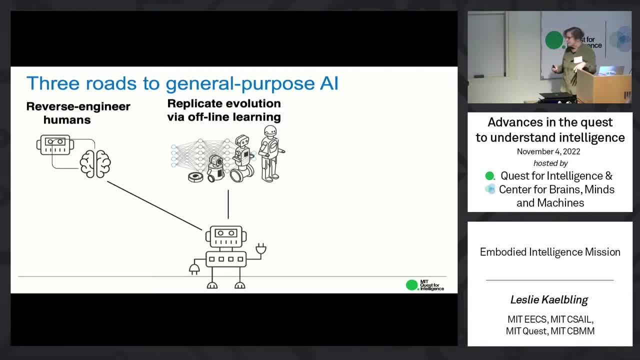 make intelligent robots that way. another strategy is, a sense, to try to replicate evolution, to do an enormous amount of work offline, searching for good solutions to the problem, maybe at this moment by training neural networks and so on, but doing an offline search for a very good behavior. and another strategy is to just use the 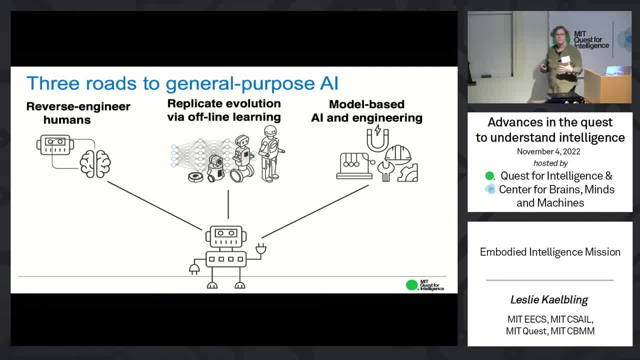 standard principles of engineering, of understanding the system that the world that we live in building, and constraints designing systems using classical methods. so all of these methods have been successful in the past in various ways. but the current research culture is kind of a monoculture and almost everybody is working on trying to build systems that search offline for a good. 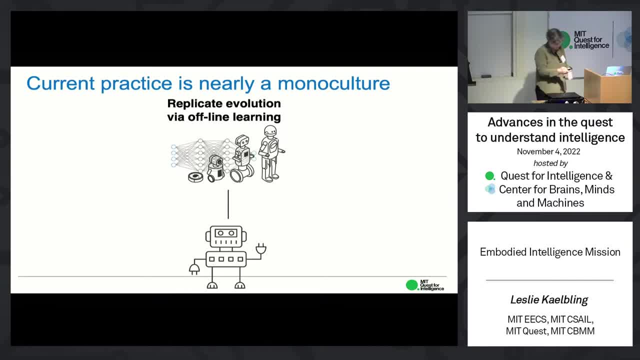 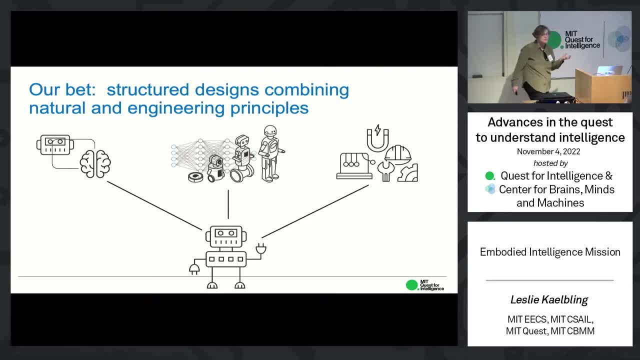 solution, like evolution searches offline for good solution that we can then deploy in the world. our bet is that actually, you do better by combining all of these three methods and, in particular, that you can learn from natural systems and that you can learn from engineering principles, good kinds of structure that 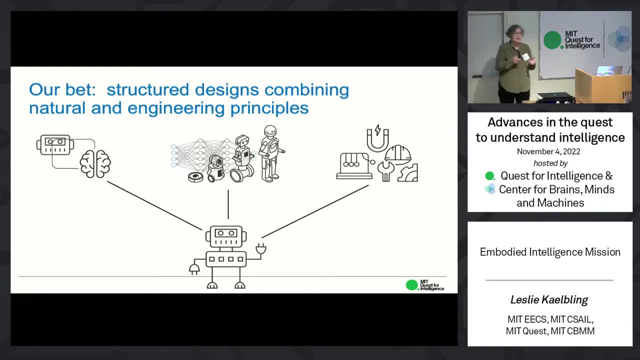 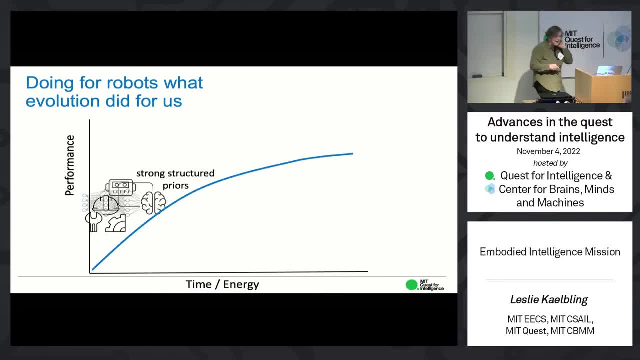 perform a substrate for doing the learning, and that can make it much more efficient. and so, if you think about it, you can see that there are a lot of things that we can learn from and that can make it much more efficient. and so you think about how much work it takes to arrive. an intelligent system, our bet. 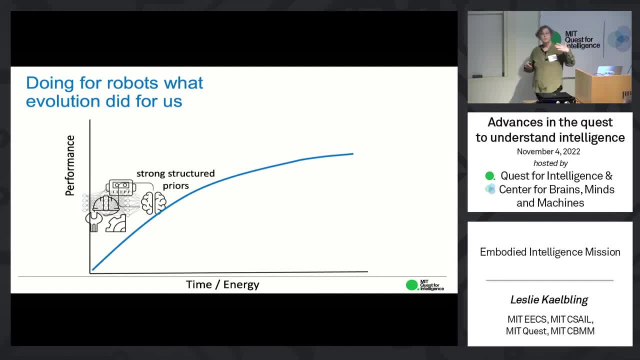 is that by building in strong priors we can learn pretty quickly as a function of time or energy or CPU cycles or GPUs or whatever, and that the approach that builds in less bias might take a lot longer, a lot more data, a lot more compute, a lot more time, although it's possible in principle that, because it. 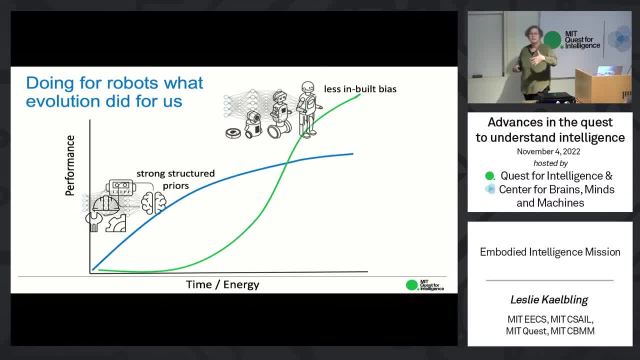 has less bias built into it, it could actually eventually learn to be better than the some, a lot more structured and design system, although we're not sure and we can't really predict where these curves are gonna cross and we're not even sure if they will cross, but it's a really interesting thing to keep in mind. I 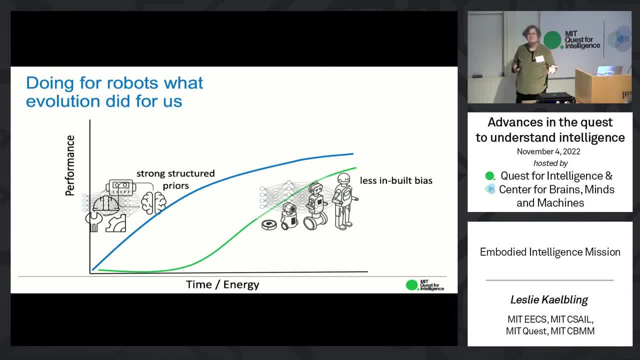 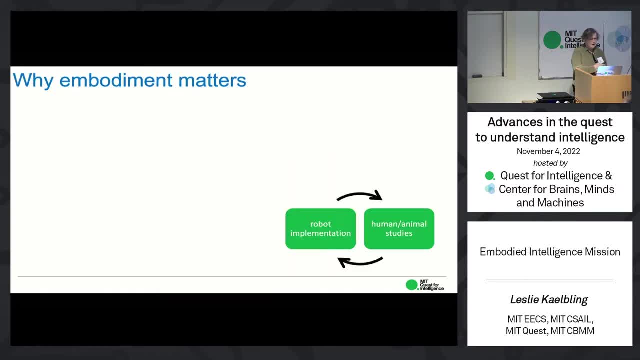 think we don't. we think that both things could work out well. we don't mean to say that you should do only one or only do the other, but that a monoculture is not such a good idea. okay, so why does embodiment matter? right, well, if you ask. 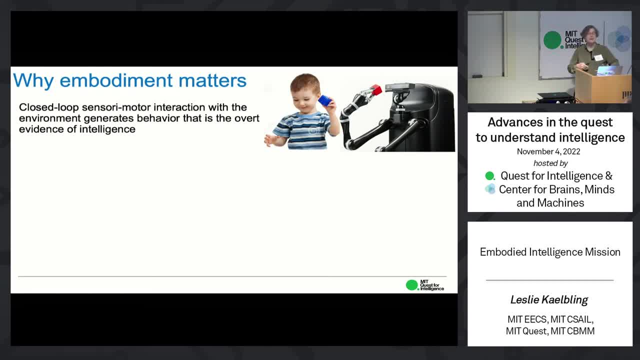 how do you measure whether something's intelligent? you look at its behavior, and its behavior comes through the inner structure of the body, and it's not just all of the body. and the inner structure comes through the interaction of the creature in this world. so our strategy is to define a broad range of 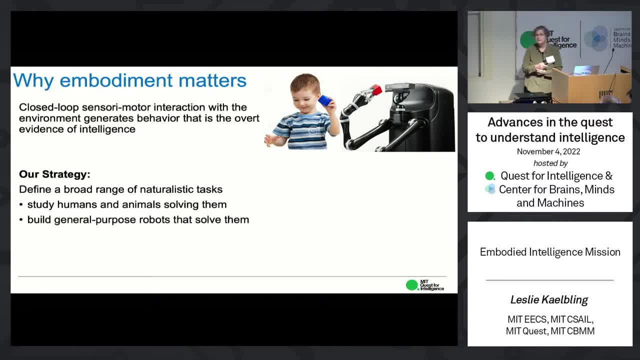 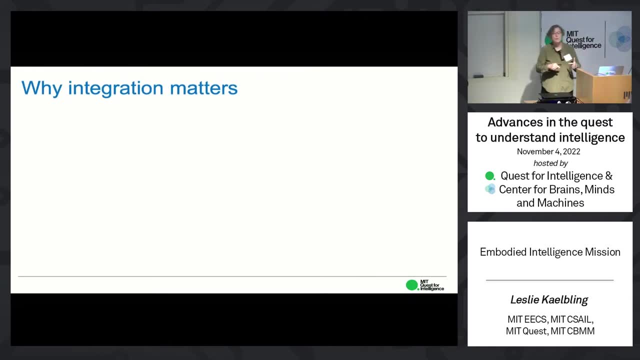 naturalistic tasks, study humans and animals solving them, build robots that can solve them too, and our prediction is that if we're asking these systems to solve similar distributions of problems, similar kinds of tasks, that will arrive at similar kinds of solutions. okay, so an important point about our approaches. 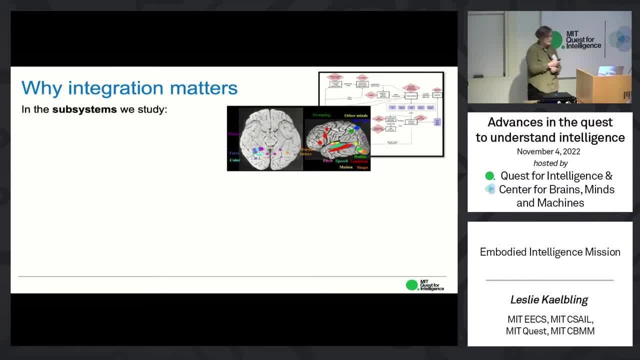 that is integrated in a bunch of different kind of ways. important kind is that we we observe in our fields, both in neuroscience and cognitive science and in computer science, that if researchers, people, tend to study little pieces of a big thing, it's easy to put your hands around a. 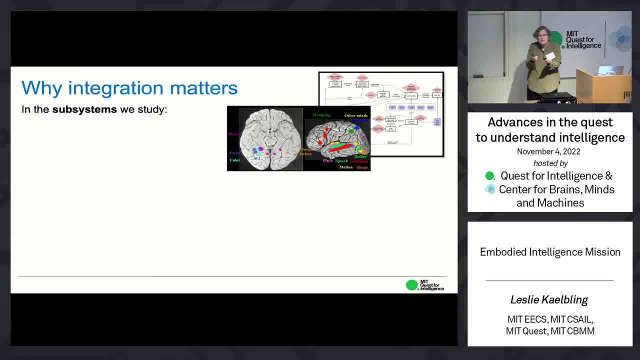 piece and study the heck out of it, but it might be hard to figure out how your piece and my piece fit together, right? so in brain science and computer science we observe that no individual module all by itself generates behavior and that to understand behavior really, and therefore intelligence, you have to. 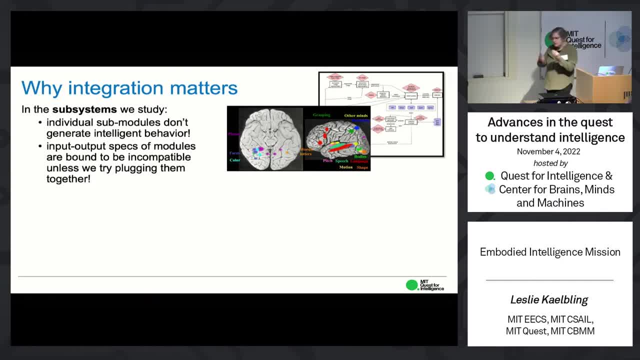 understand whole behaving creatures, and if we do them independently, we'll make assumptions that don't match, and so we have to talk to each other all the time and be sure that our parts and pieces fit together. another kind of integration is integration of methodology, so there's all kinds of different engineering. 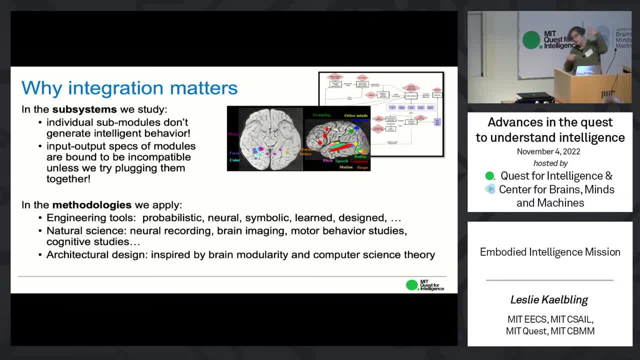 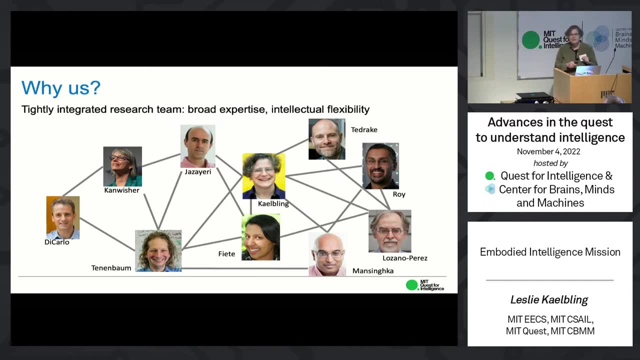 methodologies, different natural science methodologies, different ways of divining, designing structures- and we think there's value in lots of these and that, again, we have to just keep a dialogue going so that we can figure out, take the best parts and put them together in a good new way. we have a team that's very interdisciplinary. we 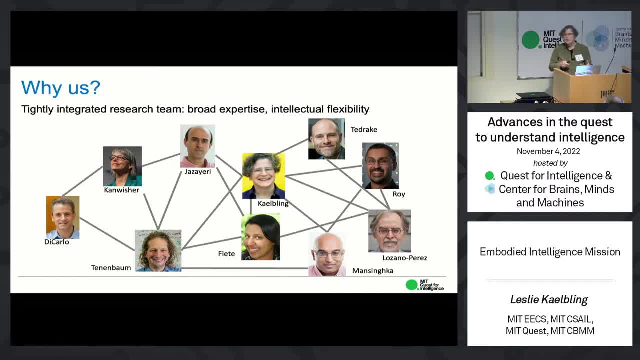 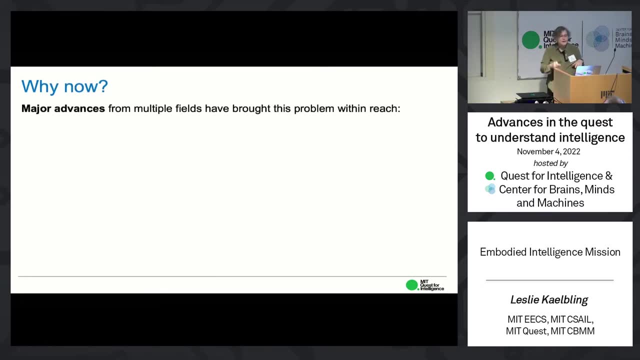 have different technical strategies, we have different foci, but we have a good property: that we like each other and we talk to each other and we work together. so the arcs on this graph are existing collaborations that we had even before this thing started. so we're a tight team that covers a lot of territory. why now? 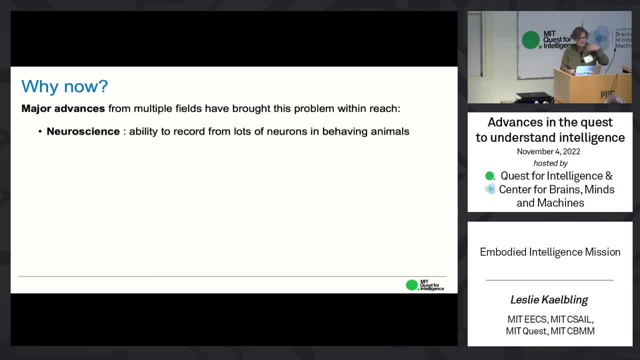 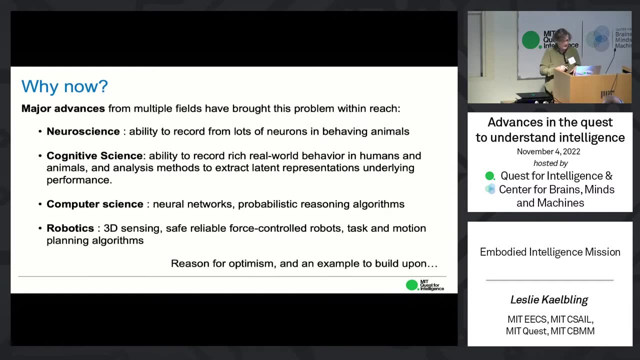 well, Josh, lots of people have talked about this already. there's been major advances in neuroscience, cognitive science, computer science, robotics, and these advances have been going on independently, but we feel like they have put us in a place where we're ready to put it all together and see where we can get okay, so we have really great. 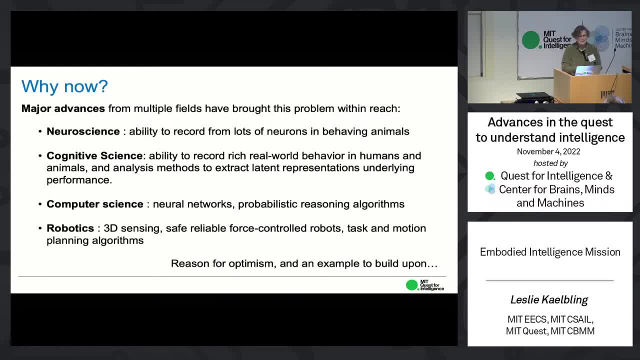 reason for optimism about this whole thing, and now my colleague Nancy is going to take over and talk a little bit about a particular example that's been very successful. so, as Leslie mentioned, I'm going to get much more concrete and talk about some, some specifics of some of the things that have already come up here. so I think 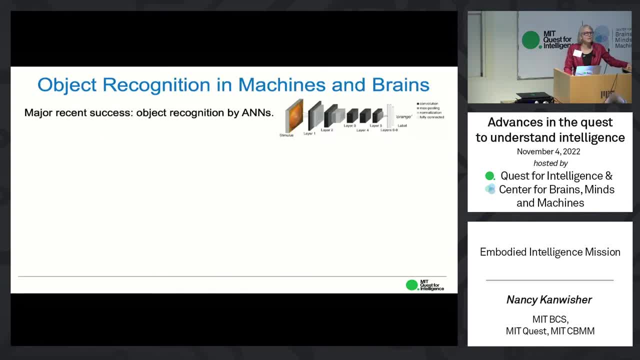 the case that's. that's really one of the great successes, as several people have mentioned in recent AI, is the ability of artificial neural networks, trained on lots and lots of labeled data, to basically be able to tell you what categories of objects are present in an image, and that's a real triumph for 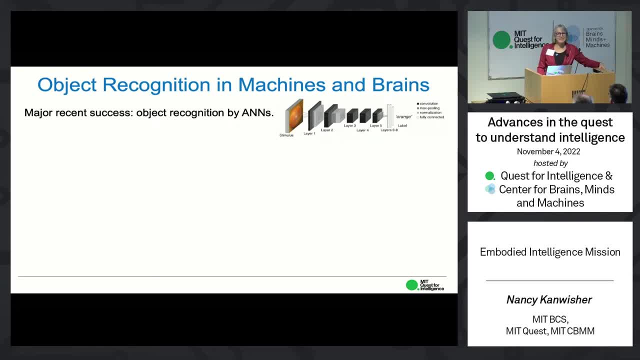 AI, but it's also very cool because it gives us concrete image, computable, computationally precise hypotheses for what might be going on in the brain. and even cooler than that. data that's already come along suggests that there are, in fact, striking similarities between how ANNs and how brains solve. 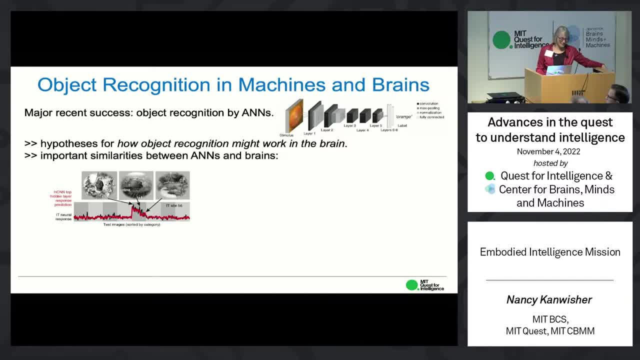 the problem of object recognition. so just as one example, in a seminal paper eight years ago Jim showed that you can actually use ANN models to make to predict how a single neuron in a monkey brain- that's part of the process of computing- what objects is in front of. 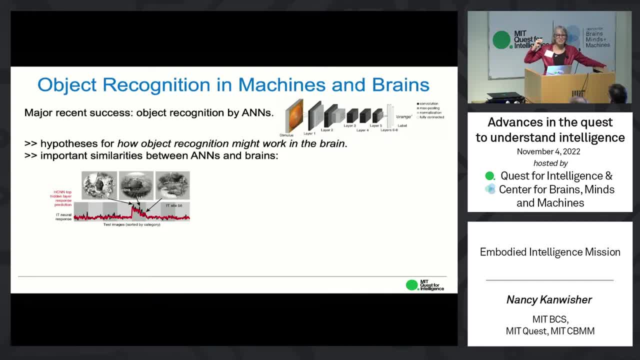 the monkey. well, how will that neuron respond to a totally new image that you haven't presented to that neuron before? so in red is the predicted response of that neuron to several hundred different images that the neuron hasn't seen before, and in black is the actual observed, measured response and you see a 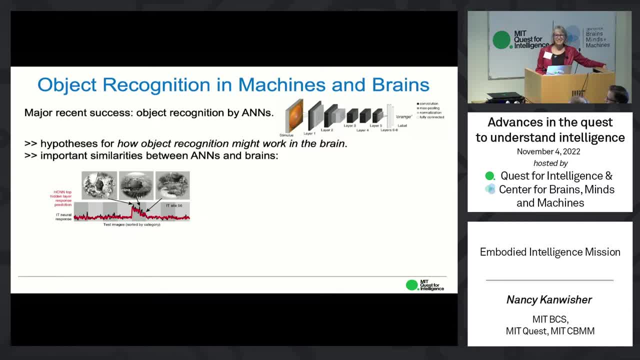 remarkable ability to predict that response and that's amazing. and more recently Jim's lab and my lab have been collaborating, actually by Ratan Murthy, who did this beautiful study over here, sitting over there, where he used similar methods to show that you can predict the magnitude of response of a patch of the 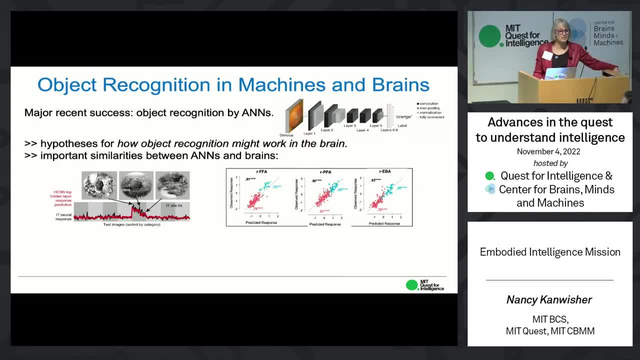 cortex in humans, a patch that's involved in visual recognition of faces and objects and scenes. you can predict how strongly that patch will respond to a novel image, and what that shows is that, in fact, brains and artificial neural networks have arrived at at least somewhat similar solutions to the problem of object recognition, and I think that's. 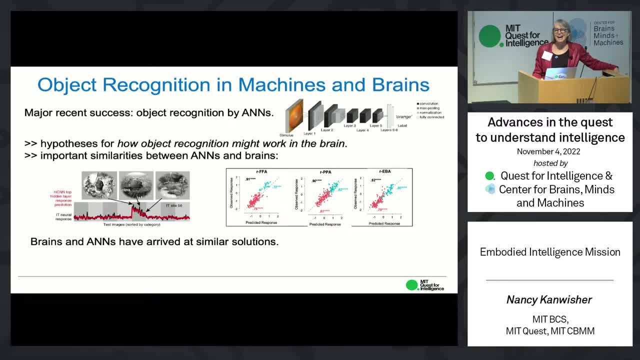 just kind of astonishing. it's so, did not have to be, and to me it's just a beautiful demonstration of something that David Marr said over 40 years ago. I forgot to put the quote in here, but it's something like: the nature of the computations that underlie perception will be determined, be determined much. 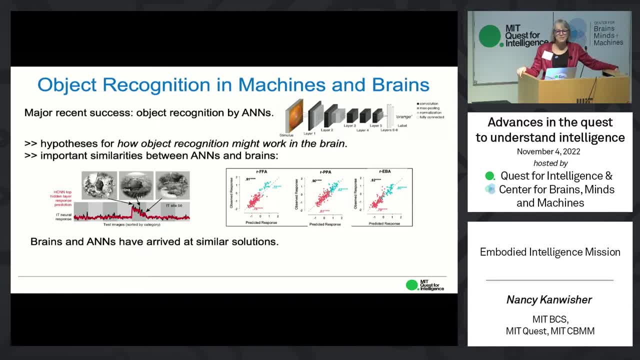 more by the structure of the task that has to be solved than by the hardware that's implementing that solution. I think this is a beautiful demonstration of that idea and it tells us that, as people have said before already today, that neuroscience and artificial intelligence have much to learn from each other. because of this, 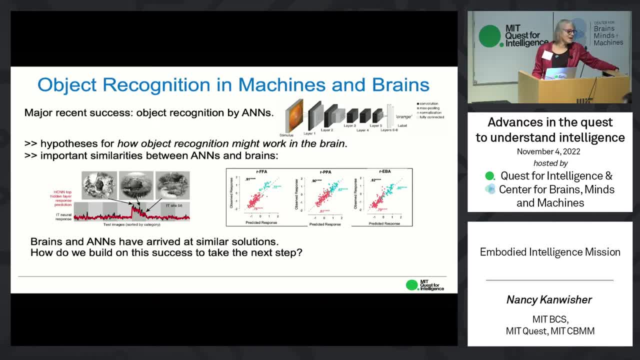 this convergence of solutions. so, as Josh and others have said, this is simply pattern recognition. this is a relatively simple problem, a teeny part of the problem of intelligence. so how do we build on this success to take the next steps, that is, to not just know the categories of things that are in front of us, but to 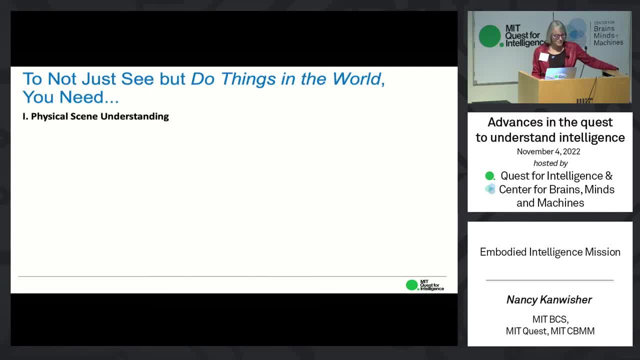 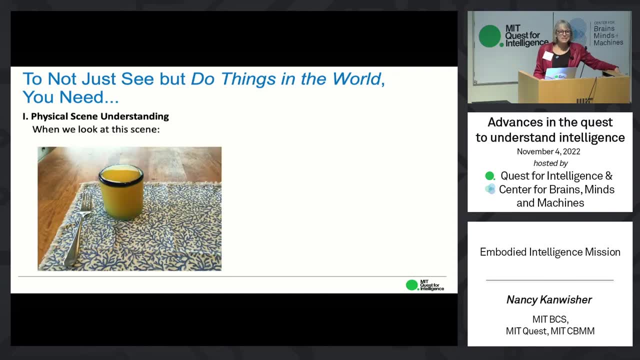 do stuff in the world, and so to do that, we need physical scene understanding. so what do I mean by physical scene understanding? well, when you look at a scene like this, the point is that you see not just the categories of objects that are there. you see that the glass is. 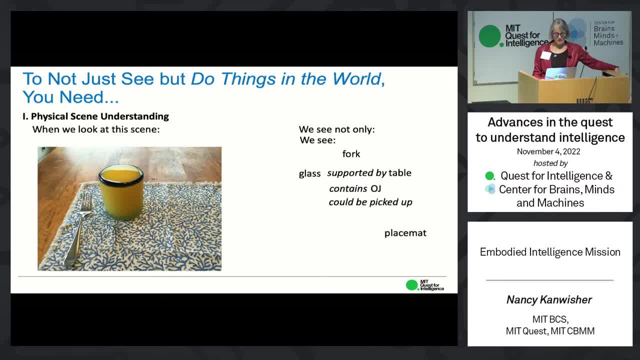 supported by the table, that it contains orange juice, that it could be picked up but might spill, containing the placemat. and you see all of that in just a few extra 100 milliseconds after that first feed forward pass delivering the categories of objects. so that's what I mean by physical scene. 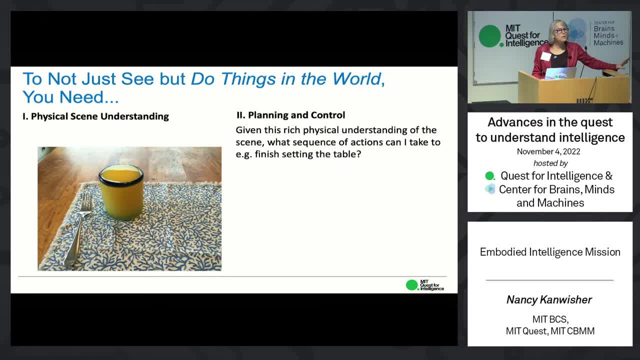 understanding and so to act on the world. you need that, but then you also need to take this rich physical understanding of the scene in front of you and figure out what sequence of actions you can take to complete some goal, like setting the table, and that entails answering some really hard. 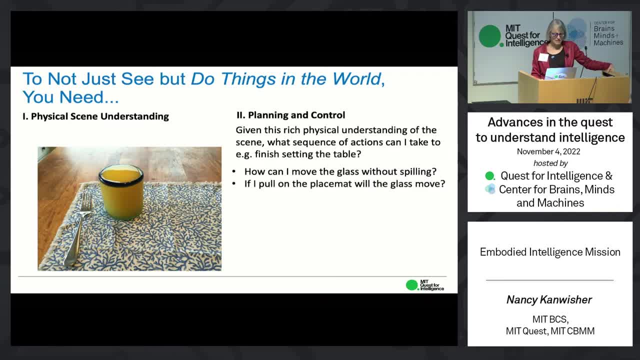 questions like: how can I move the glass without spilling? if I pull on the placemat, will the glass come along? how should I look for a plate? start at the closest place? does a human I'm serving even still want breakfast? and what should I do about that alarm I hear? so these are really really hard problems, but encouragingly our team. 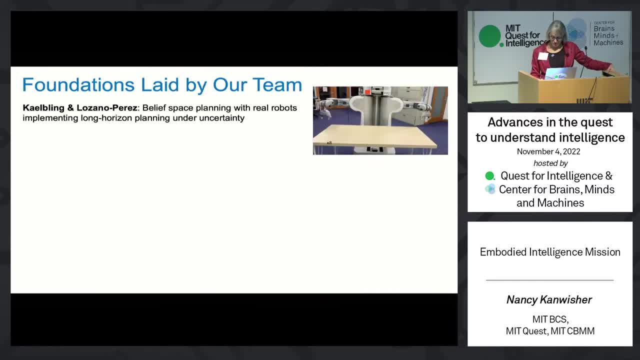 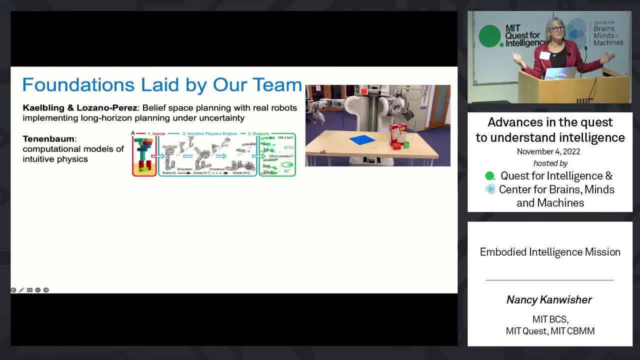 has already laid some of the foundation for this kind of work, so Leslie and Tomas Lozano-Perez have made this cool robot here. it does cool stuff by representing the belief state of the world and making these long Horizon plans under uncertainty. Josh Tannenbaum has devised these computational models of physical scene understanding, in which 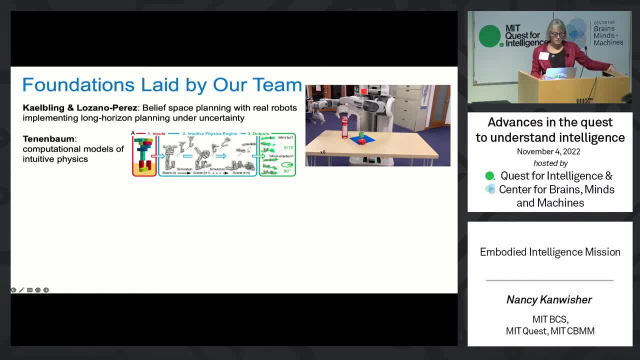 you start with an image, extract a representation of the physical structure of the scene, use a forward physics model that predicts, time point by time point, what's going to happen next. and he's tested that model against humans performing the same tasks and found remarkably good fit between his model and what humans do. and Vikash Mancinga has developed these amazing computational 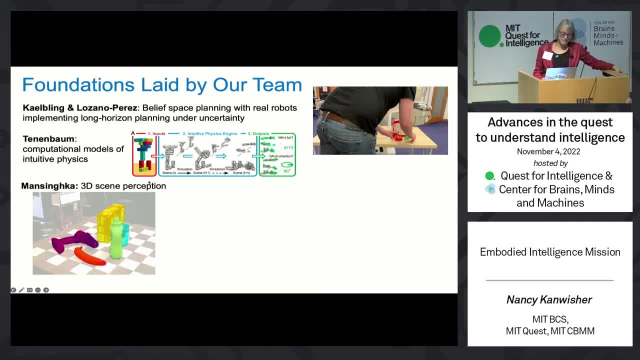 models of 3D scene perception that can segment, segment objects in the image, figure out their 3D shape and figure out what's touching what. in collaborative work between me and Josh, we've identified some candidate regions in the human brain that seem to be implicated. 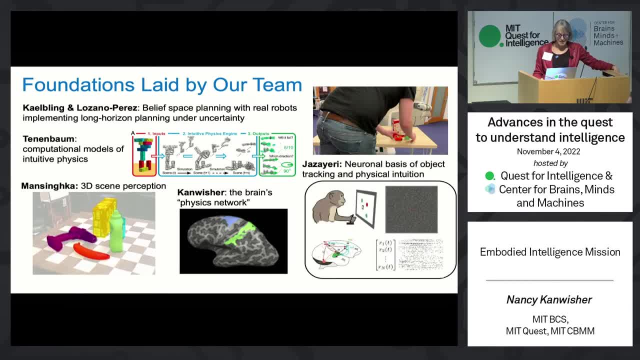 in physical scene understanding, telling us where to look in the brain- who will be speaking in a couple minutes- is looking at the neuronal basis of object tracking and physical intuition. So to take the next step, together we're going to tackle a concrete but broad class of problems. 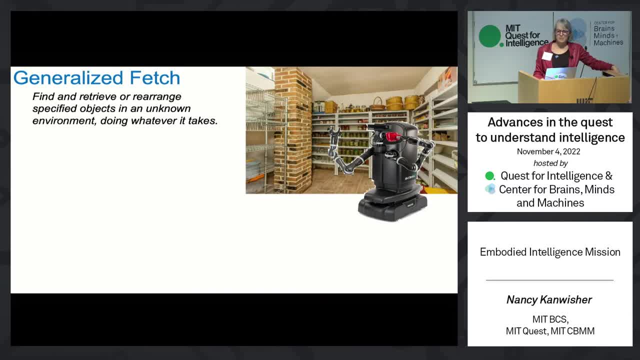 That's known as generalized fetch. That means find and retrieve or rearrange specified objects in an unknown environment, doing whatever it takes. And why is that a good problem class? Well, for a number of reasons. One, it's actually a huge space of problems and we want to have one solution that solves. 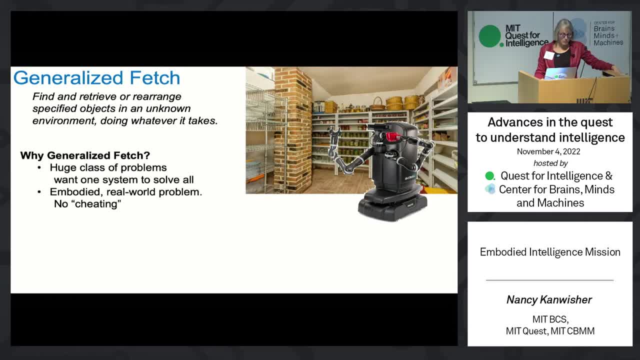 all of them. Second, it's a classic embodied real world problem. You have to go all the way from perception through to action. You can't cheat and skip a step. And third, it far exceeds the current state of the art in both what we understand about. 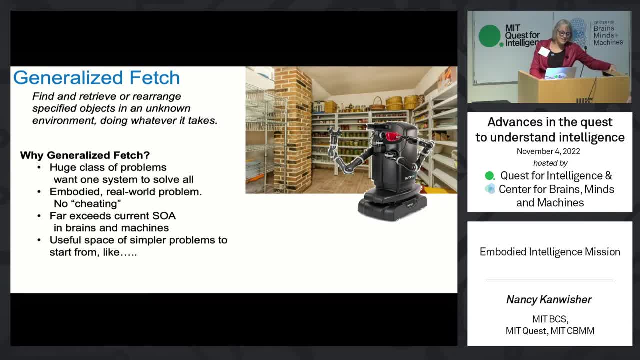 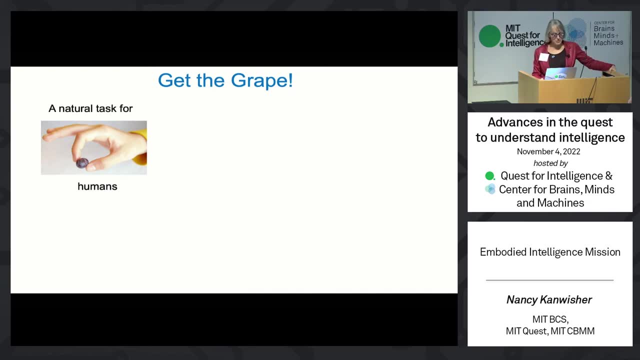 brains and what we can do in machines. And, finally, it has a useful, simple space to start from, from which to begin To build, And the simple space we're going to start from is a task called get the grade, And this is a very natural task for humans, for monkeys and for robots. 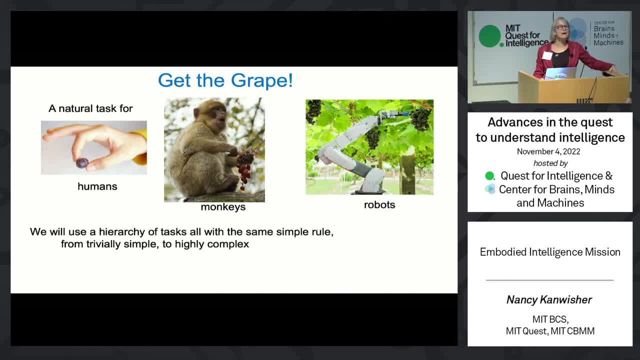 So we're going to do this in all three of them and we'll start with a hierarchy with some very simple tasks scaling up from there from trivially simple to more complex, And for the human version of this task, we're using a simulation platform devised by engineers. 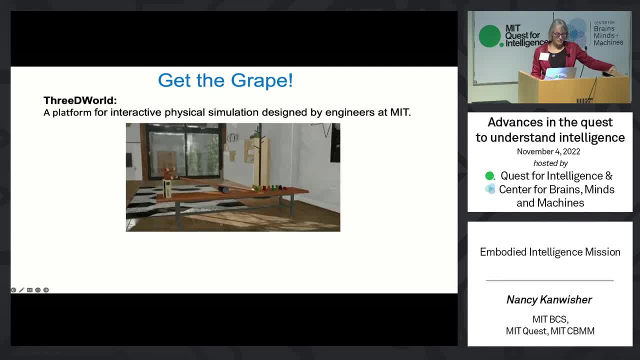 here at MIT called 3D World, And it can create these beautiful, very realistic renderings of worlds And it can simulate physically what's going to happen in those worlds. So, for example, if you perform an action on it, it will give very realistic forward, physical 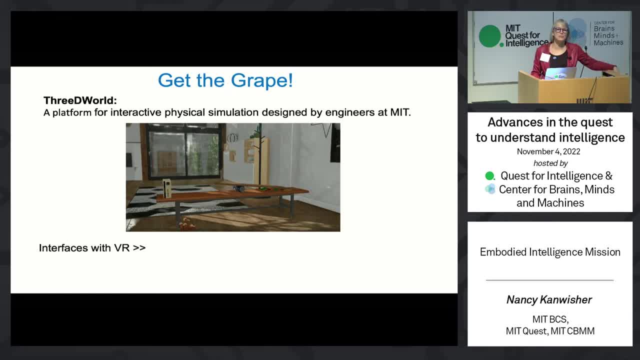 simulation. But also importantly, it interfaces with virtual reality so that we can put a human in a VR space and give them an action task and record all of their behavior, from eye movements through trajectories of hair, So we can measure how people perform these. Find the Grape tasks. 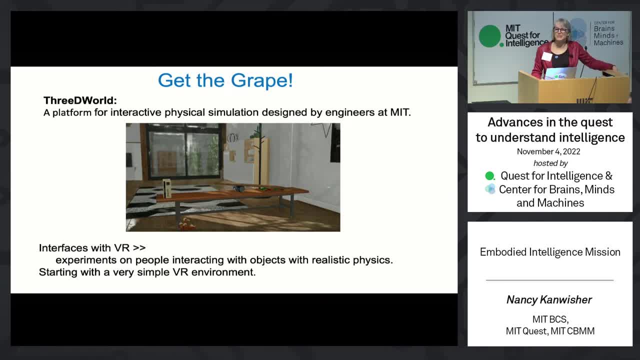 And so we're starting with the simplest and most rudimentary versions of this Get the Grape task, And to do that, we're going to show you a very simple example of this, and we're going to ask Jim to get the grape performed by Arian, who's going to put him in VR and get him to. 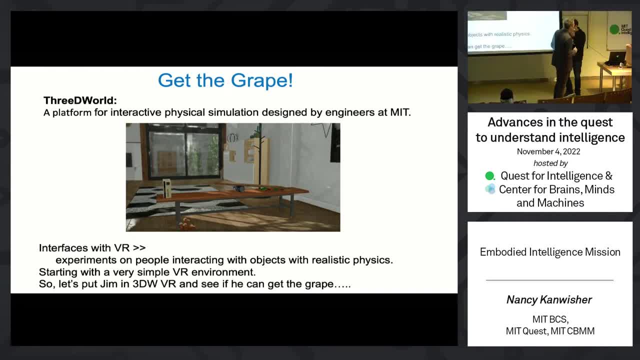 find it. See if he can find the grape. So we designed it. So there's a couple of very basic, rudimentary tasks And we're going to show you a very simple example of this. So we're going to show you a very simple example of this. 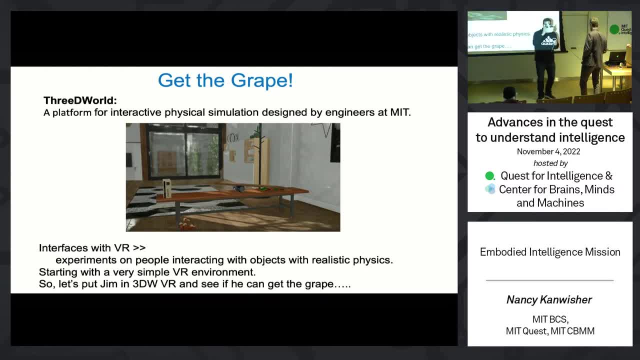 So we're going to show you a very simple example of this. So this is a very simple example of this. So a very simple example of this. This is a very simple example of this. Jim is going to put in a rudimentary task and then a more complex one. 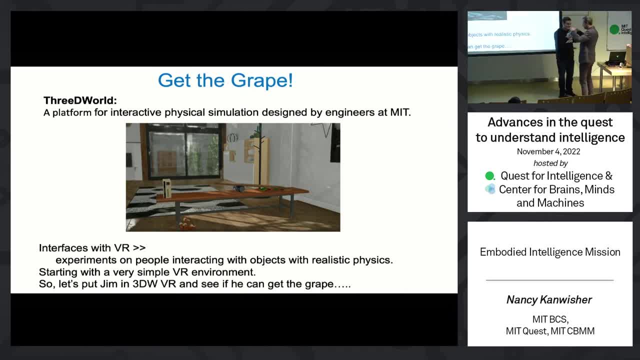 We'll see if Jim can do that that he hasn't done before. Yeah, this is scary. I'm scared that the director of the Quest for Intelligence is going to look non-intelligent. What am I doing? So this is what Jim is seeing. 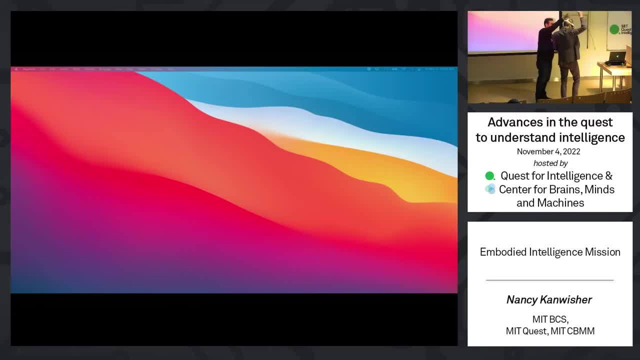 Wow, So he's got to get the grape. The grape is somewhere, The thing doesn't move. If he tries to move you, the first thing it does is move the grape. Oh, wow, So that's what Jim is seeing. 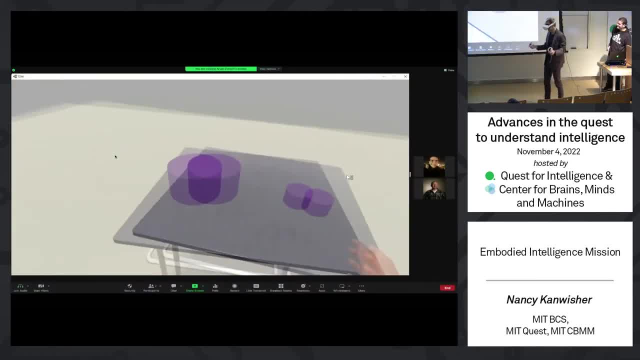 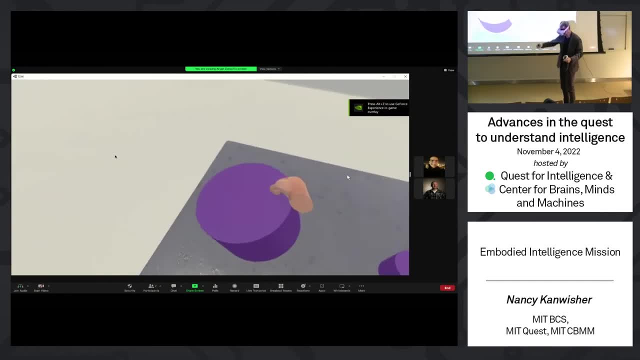 what am i doing? so this is what jim is seeing. wow, so he's got to get the grape. grape is somewhere, the thing doesn't move. he tries to move the first thing, it doesn't move. all right, go jim, okay. okay, that was pretty basic. let's do another basic. oh, i thought i succeeded. 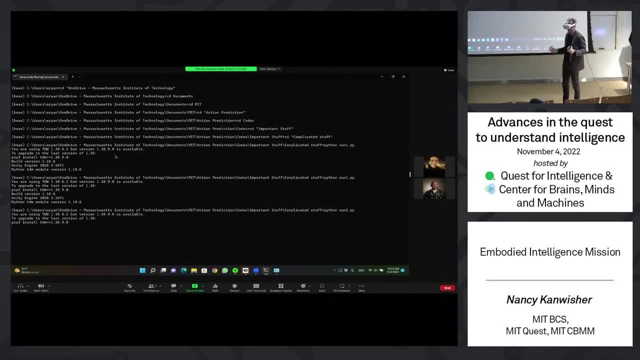 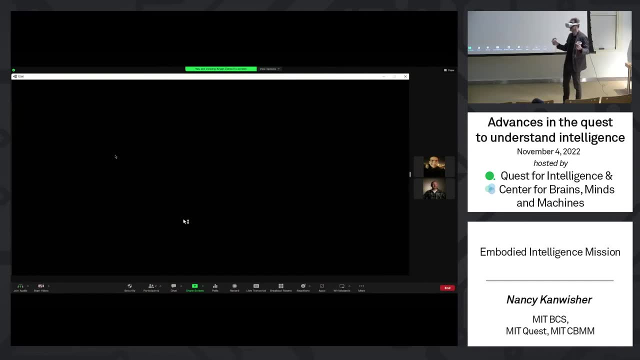 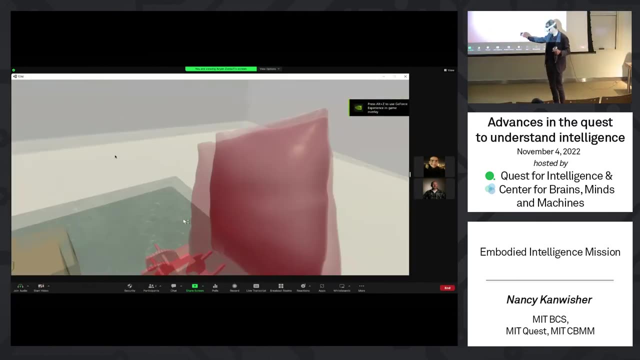 okay, no, that was the easy one, jim. all right, that was the easy one, okay, yeah, okay, do i clear this? uh, what's happening? it's taking, here we go, here we go. oh, there's stuff. okay, all right. are you guys seeing all this? jim? you're making a mess, throwing stuff all over. 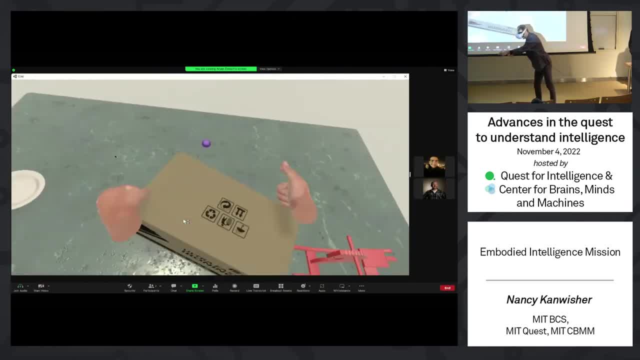 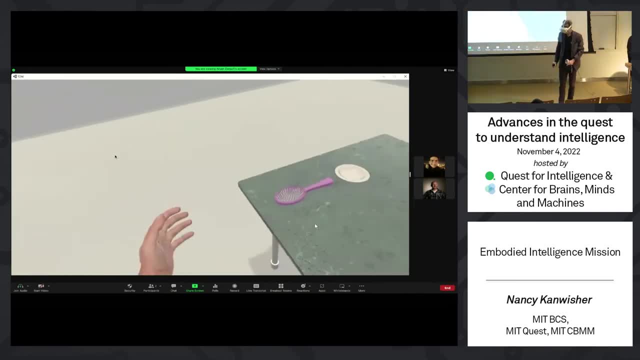 clean up your room. i thought i was supposed to be like a four-year-old, okay, so oh, there it is. yeah, that's no problem, all right, go jim. yeah, all right, all right. the next one: we designed to be more like jim, and then jim was like jim, that's, more like jim's sister. 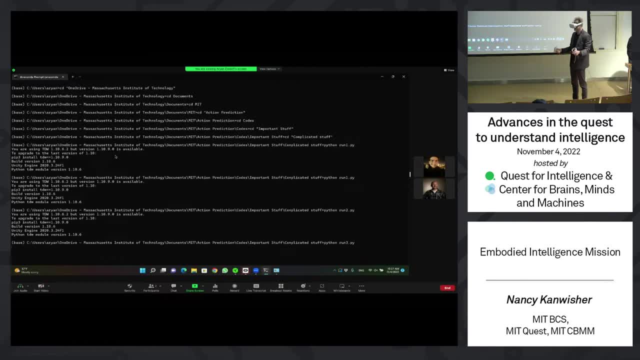 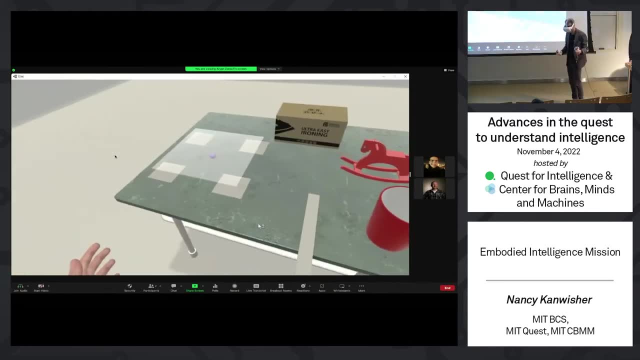 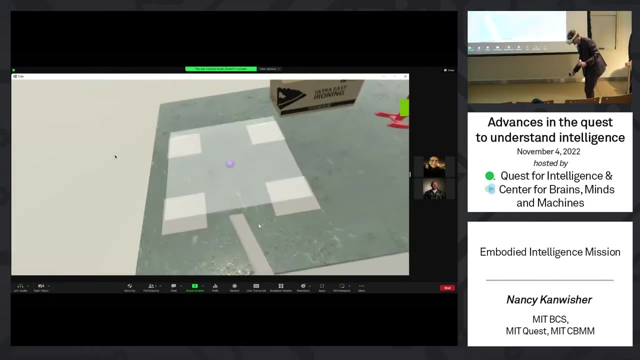 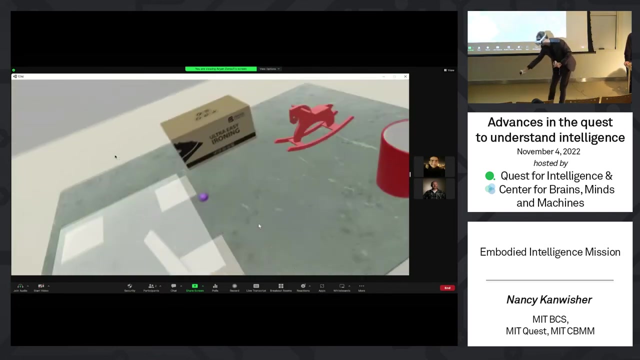 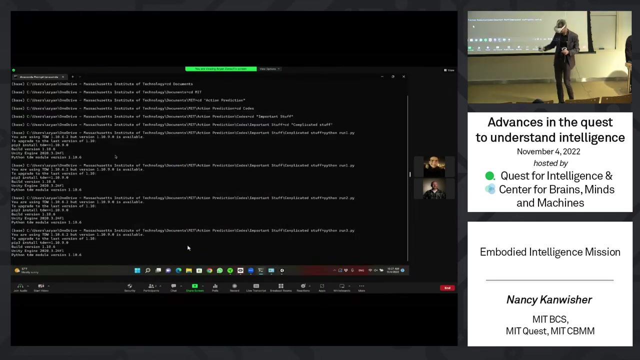 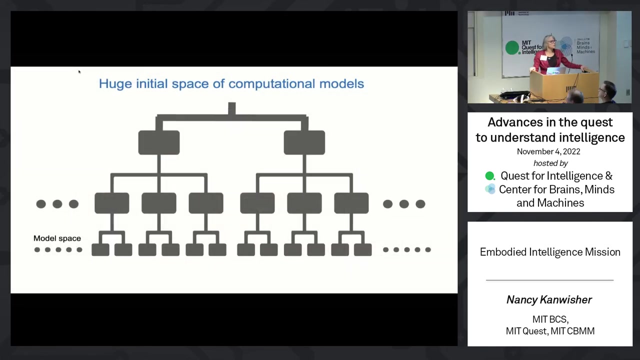 more tricky. it involves, like, some significant innovation, so who knows if Jim will be able to do this? he hasn't seen it before. okay, okay, oh, that's all right. I think I know what you're trying to get at. okay, great, thank you, that was wonderful. you did great a plus. so the 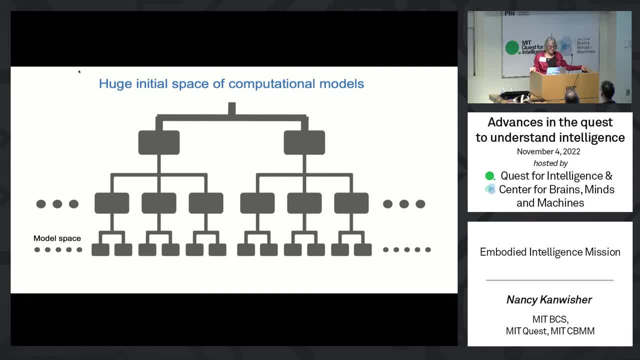 question is: how did Jim do that? that was amazing. that was awesome, but there's a huge space of possible computational models for how he might have done that, and so, by collecting rich behavior, old data, we'll be able to prune this tree of possible computational models, but only partway. we'll still be wet, left with lots and lots of possibilities of. 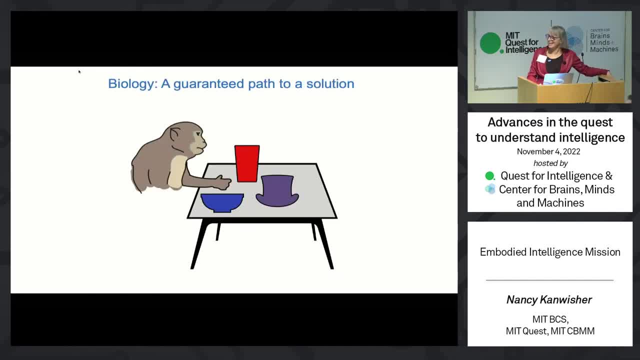 what algorithms might be running in his head when he's doing this task, and that's why we need Murdad and his monkeys. she learning in limited domains, but when it comes to real-world tasks and real-world environments, we don't have good solutions currently, and the monoculture is such that we might not. 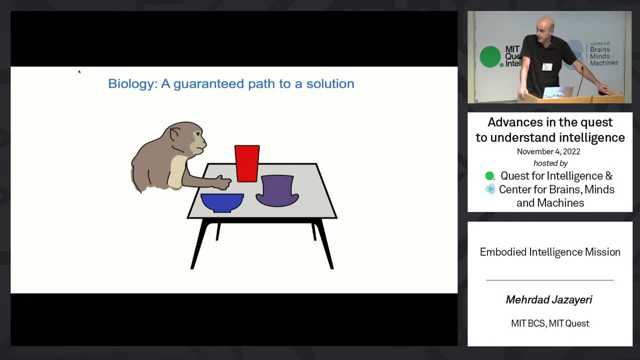 actually even know what we're doing and we don't know what we're going to do, so we need to find a solution. if we just continue on that path, well, that said, we know that there exists one guaranteed path to a solution, and that's the brain. 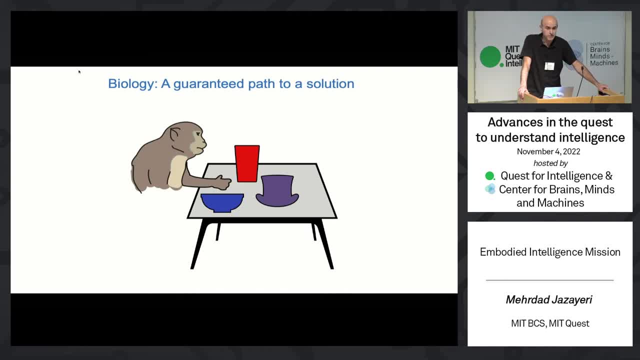 we know the, the brain kind of offers the kind of intelligence we're looking for. so if we were to to understand how the brain solves it, we would have the solution in our hands. in my lab we work on non-human primates- macaque, monkeys- to study their brain, to try to understand how they 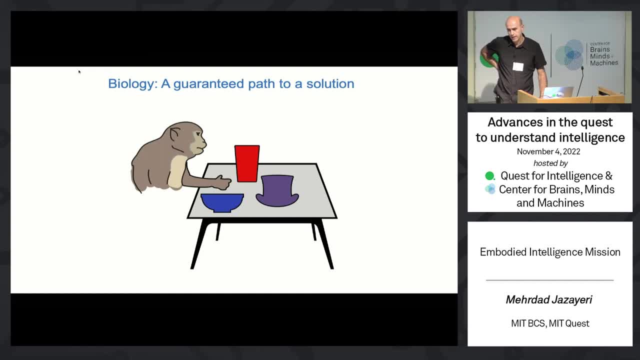 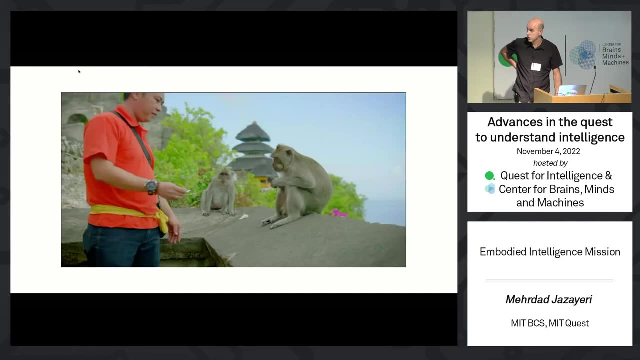 develop intelligence. now in for those of you who are not familiar with this kind of work, you might think: like: what do monkeys have to offer to this process? and I want to share with you three points. point number one is that these monkeys actually are quite intelligent. now I'm going to show you a little fun video of. 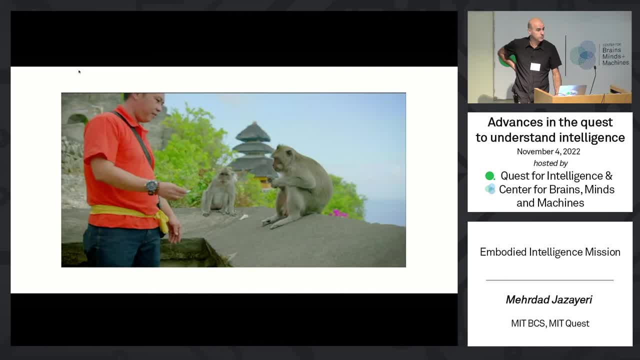 monkeys trading objects with folks that are nearby. you'll see them handling object, but more importantly, you see that they are intelligent and that there's even more complex factors. Yeah, I've been carrying them lately, but that's a great question. That's a really early aspect. 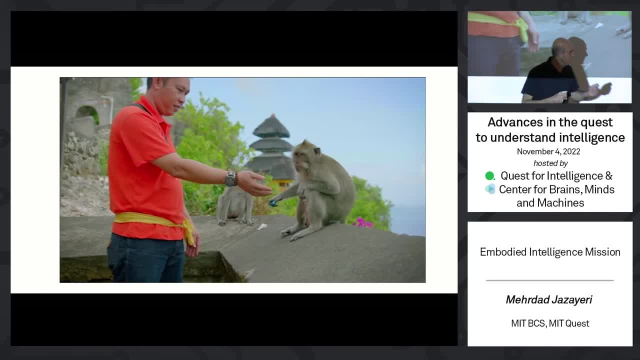 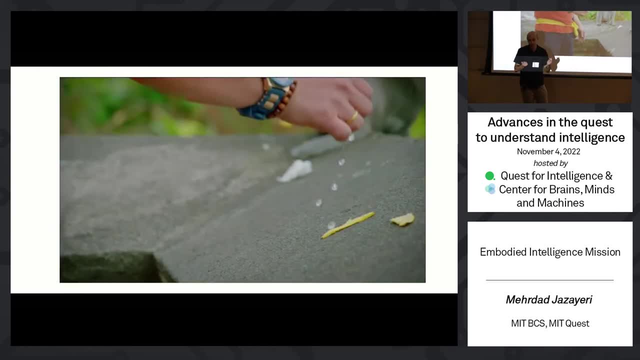 indeed intelligent. now what you will see is that these monkeys steal the glasses and various objects of people, right, and they go somewhere and they wait until the person figures out: okay, i need to give this monkey something. they don't like the the glasses, of course, but they want food, they want. 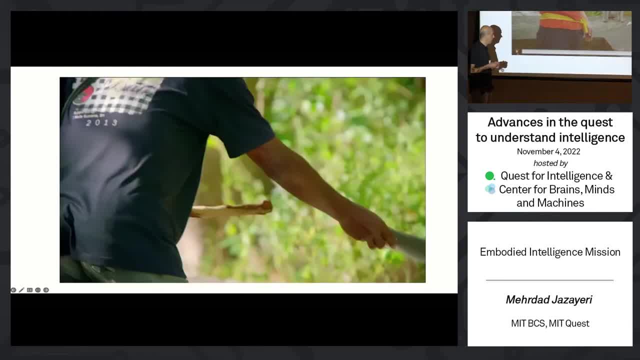 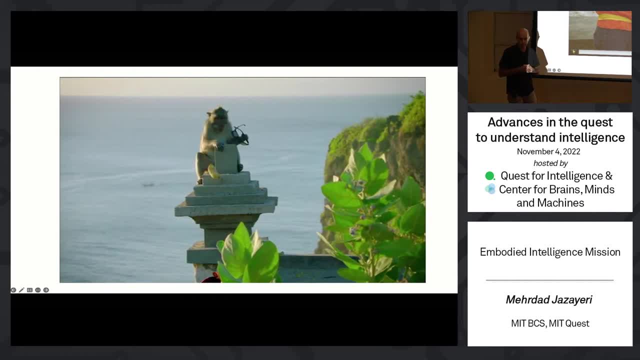 bananas. they want something else and what happens is that they wait for a while and until they basically- you know they're testing the human intelligence there- that are you going to figure it out that i want your banana? and at some point people figure it out and they give their banana. 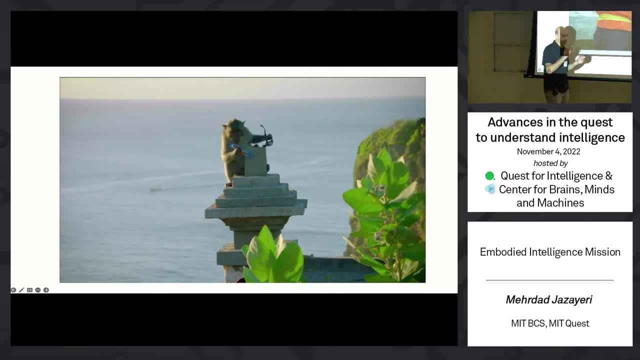 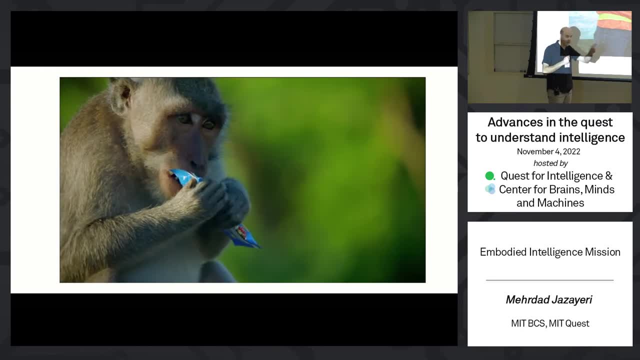 and then they quickly get it and give back the object. and they do that. they wait until they get what they want. so if you give them what they don't like, they refuse. it's like: no, i'm holding the glasses, i want that other thing, i want the candy, and they do that and they get it. so you get a. 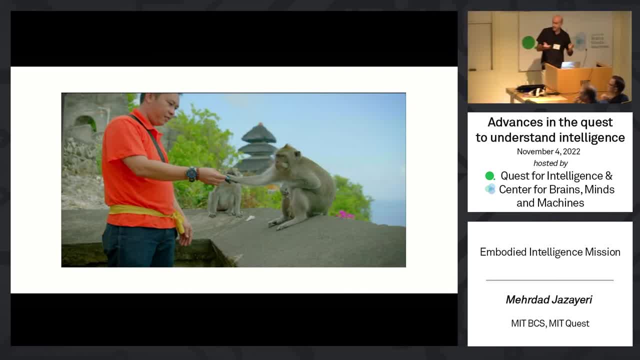 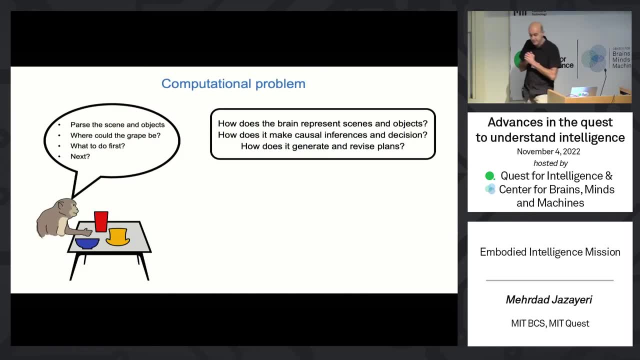 sense that they're quite intelligent. they are they, you know, they understand social interactions and they can handle objects. so that's point number one. they're quite intelligent, so we can study intelligence in these animals. point number two is that we think we have found kind of the secret. 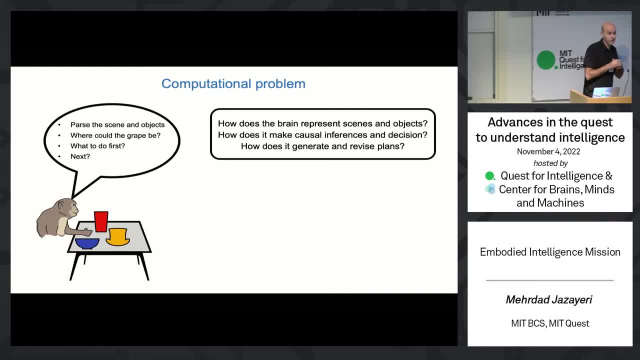 sauce of how to well this was in their natural habitat. but we think we have found kind of the secret sauce of like how to bring this kind of intelligence into the lab, setting any guesses on what that secret sauce is. well, remarkably, it's actually embodiment. so what we have found is that 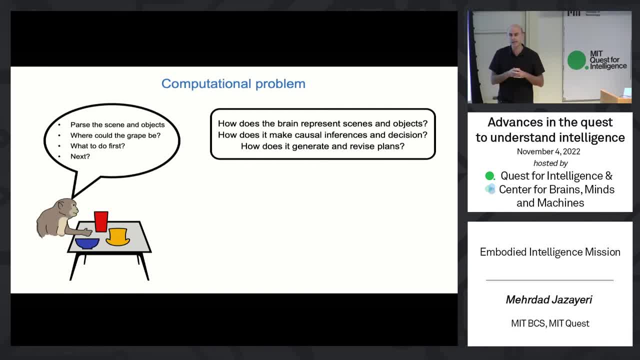 when you put these monkeys in front of a computer monitor, a screen and a joystick and such, they often find contrived solution to the problems that they don't generalize well, they're not quite flexible and they're not able to really take advantage of their knowledge and intelligence. 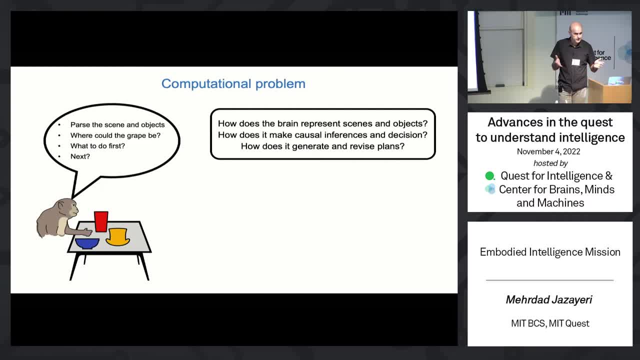 on the contrary, when you put them in front of a tabletop with real objects, they quickly reveal that they understand objects, they understand the relationship between objects and they know what they can and cannot do to those objects. so they they very quickly kind of express what you know over the evolution they have learned. 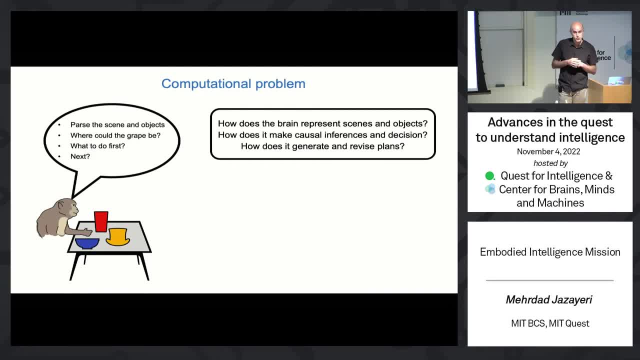 to do in the settings that are real. so we're going to have a version of the uh get the grape for them, which is with physical tables and physical grapes and physical objects, and what we hope to do is to use that setting and the animal's natural uh embodied intelligence to 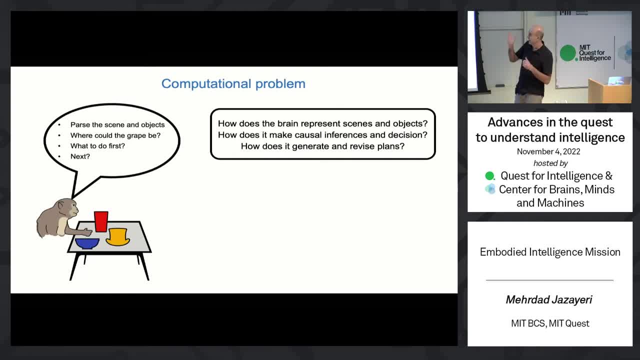 ask questions, fundamental questions about intelligence, like: how does the brain represent objects, how does it make causal inferences, how does it make plans to interact with the objects and revise those plants? uh and uh, the plan is to, of course, while the animals are doing this, to record from their brain. but the um setup of the get the grape for monkeys introduces some major 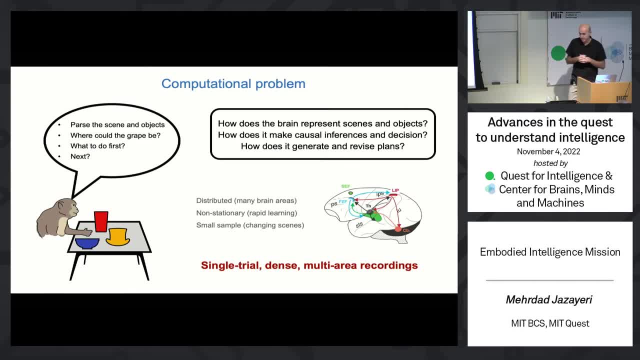 challenges. first of all, as uh, leslie and nancy mentioned, this is a integrative problem. it requires multiple faculties- perception, memory, cognition, action- and that means that many parts of the brain are going to be involved. so we need to be able to record from multiple parts of the brain. 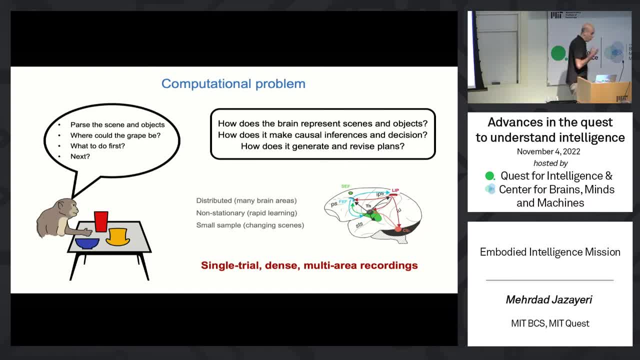 simultaneously. in addition, a hallmark of intelligence is that you learn very rapidly and you can very quickly generalize to very novel conditions, and what that means is that we ought to be able to record from many, many neurons simultaneously within single trials. we need to capture the animal's mind as it's thinking about it and we need to be able to record from many, many. 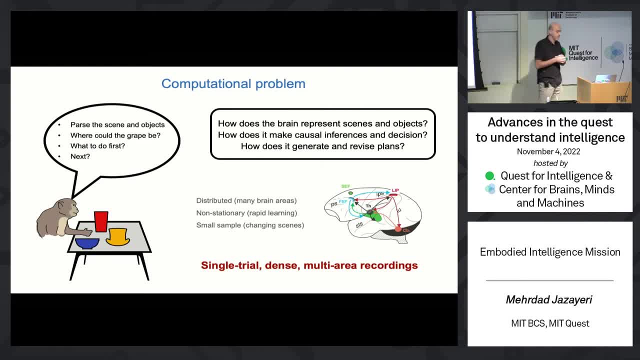 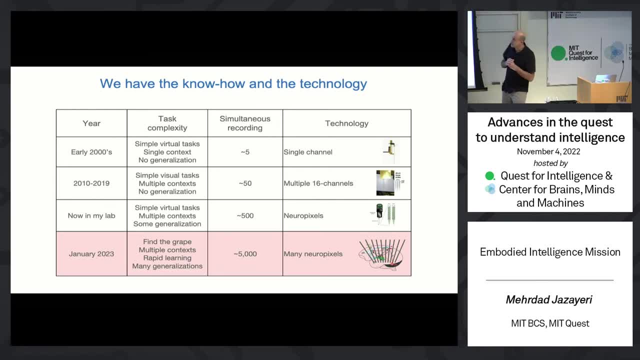 neurons simultaneously within single trials. we need to capture the animal's mind as it's thinking about a new condition, right as it is doing that, right. so, and that brings me to point number three. as you see, in, you know, early 2000, when i was a student, we could record from a handful of neurons: 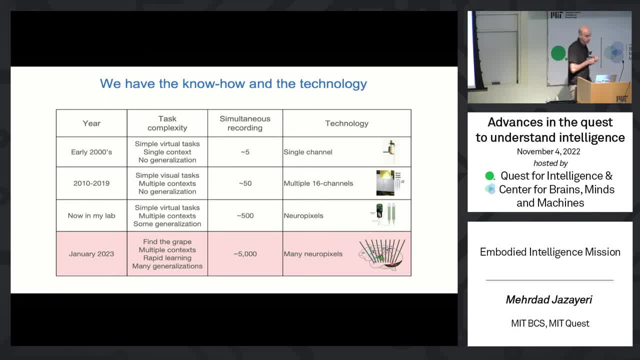 simultaneously. in the past two decades we have come a long way. that has increased by two orders of magnitude and currently in my lab we're setting up to record from a few thousand neurons simultaneously and we think that puts up, puts us in the right sort of ballpark to be able to begin to. 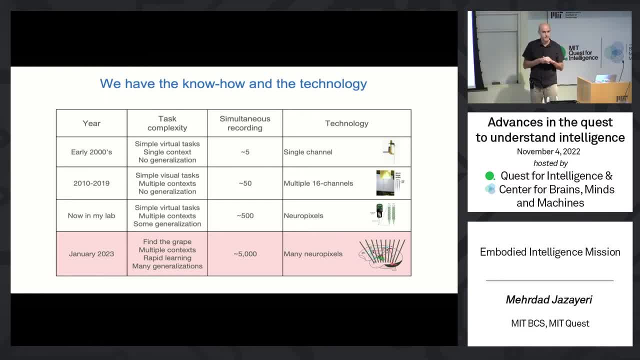 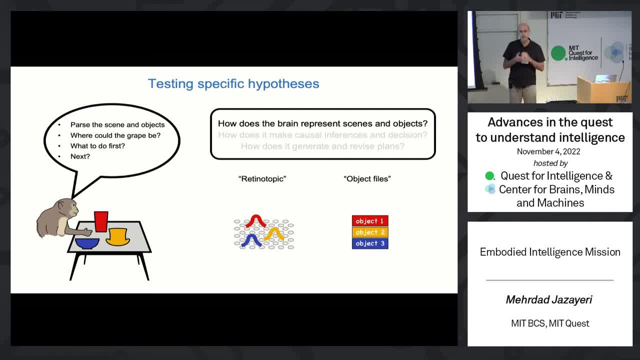 think we can then analyze them and extract from them certain various hypotheses and uh possibilities of how the brain solved this. for example, if we think about the object representation, we can look at the neural activity to see to distinguish between whether the object representations are retinotopic, which means the object representations are retinotopic and the object representations are. 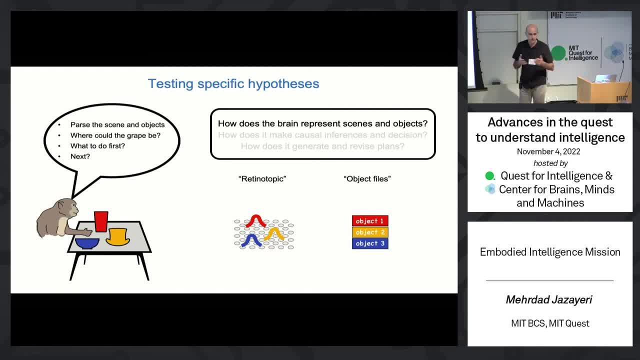 tied to space or object files, which is inspired by theorizing in cognitive neuroscience and and computer science, uh, for representing objects and if we were to find, for example, or another example? similarly, you know, we can look at the structure and dynamics of neural activity as the animals. 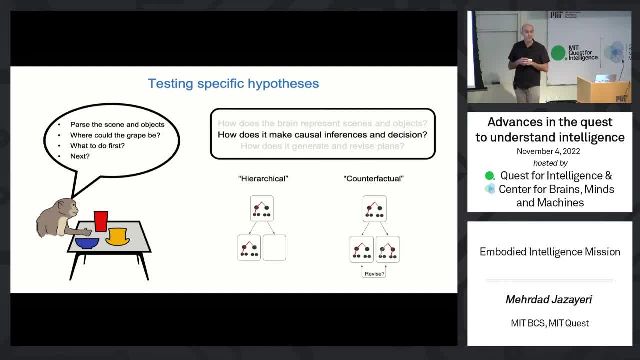 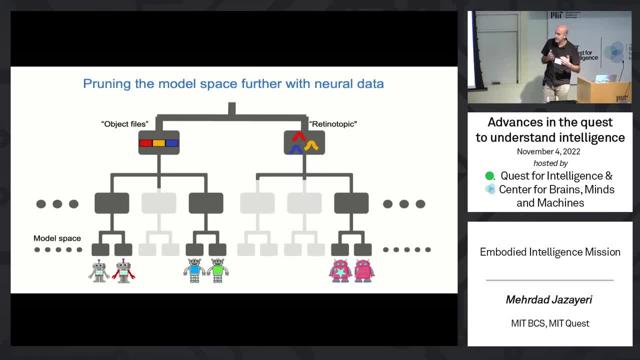 thinking and interacting with the objects to infer the strategies that they might be using for making causal inference okay. and if we were to find, you know, one of these is turns out to be the situation. so, for example, for object representation, we can look at the structure and dynamics of the 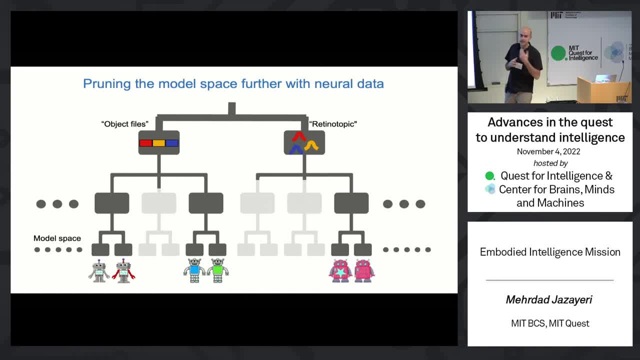 object representation. if it turns out that the monkey's brain uses a representation that is more aligned with object files compared to retinotopy, that will allow us to further prune, further constrain the search to sub branches of this, uh, this tree, and uh, help you know the, the larger. 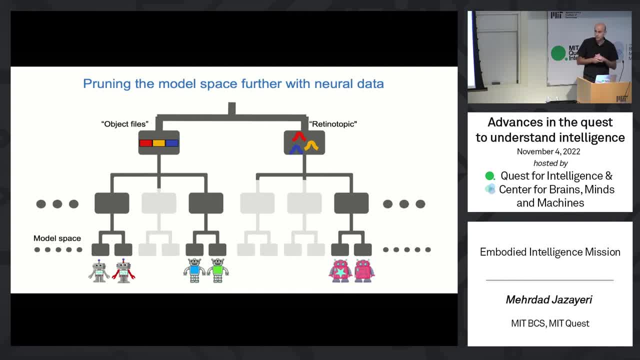 tree that are trying to figure out how to build models, out, how to uh sort of integrate, uh to make a much more efficient search and hopefully make the curve that leslie showed you bring it further down and down. so quickly we get to the answer and with that i guess i'll pass it on back to leslie to. 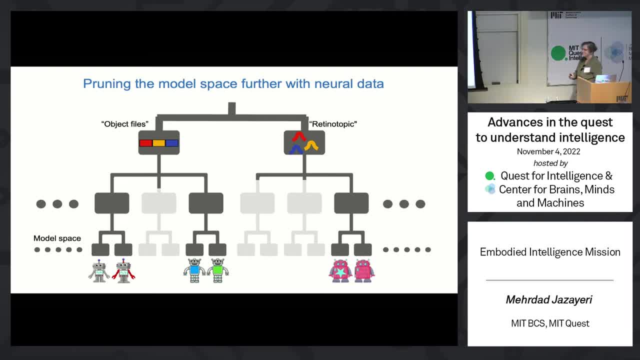 tell you how, uh, we hope to use this information to engineer next-gen robots. all right, so here we go. we, uh, what did we do? we started with a big hypothesis space. we pruned it based on behavioral data, let's say from humans. now we can prune it further based on, uh, actual neural recording data. 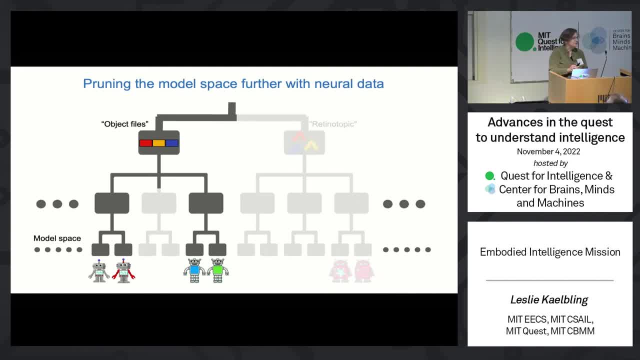 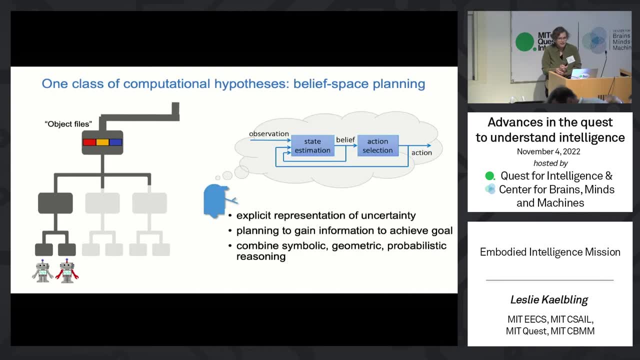 for monkeys. um, so maybe now we we're down to a smaller set of hypotheses about how things might go. now we can try to test some hypotheses in a robot and so, for instance, i might take a particular class of algorithms. in this case i'll talk about uh, algorithms, that plan. 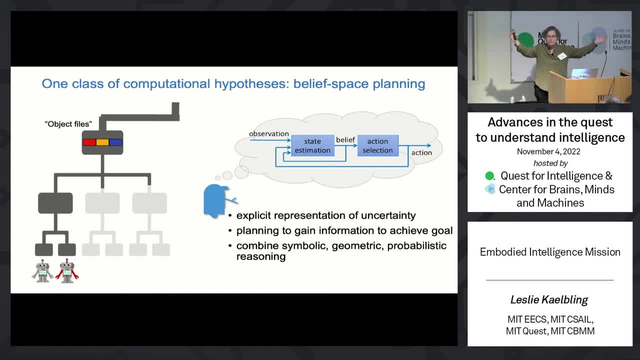 in belief space, that where we divide the problem of thinking about the world into some building a representation of what we know about the world and actually explicitly our own uncertainty, and then the problem of taking that uncertainty and deciding how to behave. so that's kind of a class. 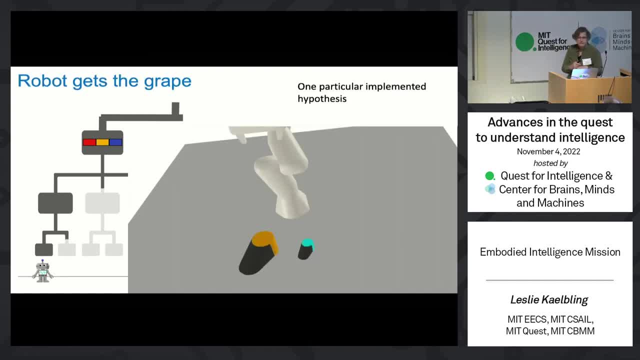 of controllers for robots, and then we're going to take a particular class of algorithms and we're going to take a particular class of algorithms, and then i can actually go further and take a specific one, so a particular implementation of a particular instance of that category of algorithms. 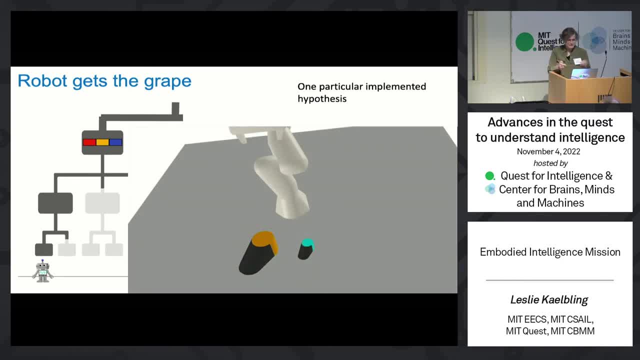 and gather data. now we'll see. probably the movie might. oh okay, good. so here we have the robot in the same setup. it's looking for a grape, uh. it tries to move that object and it can't. it tries to move this other object, thinking that the grape might be underneath there. it has moves. 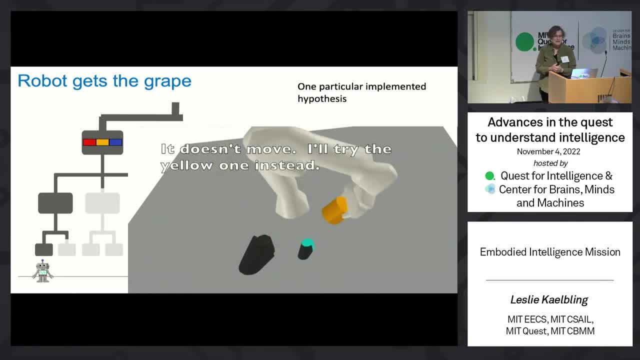 it carefully so that it doesn't disturb whatever is underneath. um, uh, and it looks to see now it. we simulate, looking right now at the moment simulated- and we find another object there, not the grape, but if the object could still maybe contain the grape. so the robot is reasoning about. 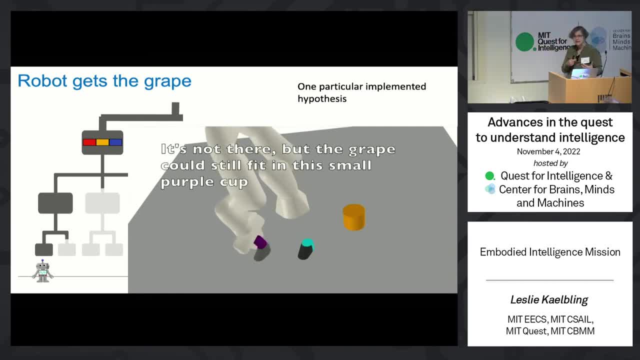 where? what parts of the space has it not yet seen and it explicitly plans to look in places that it hasn't yet seen. and these glosses that we have in the movie are actually. we can find nodes in the search space. we could build visualizations that would help actually understand. 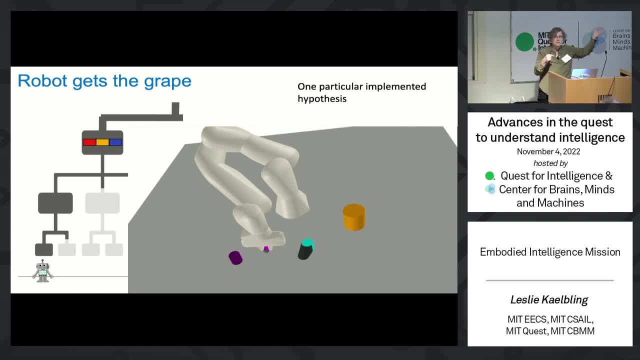 what the robot's thinking while it's doing this. so it finally picks up the last little cup and it finds the grape too. the robot is probably not as happy as jim or the monkey about having found the grape. we have to work on that part, but still, if we tell it to look for a grape, it will okay. so, uh, we. 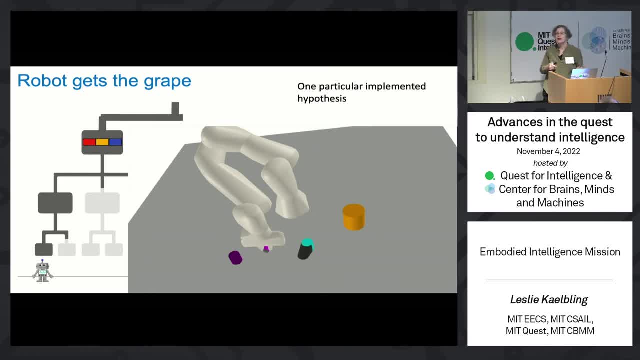 can. then, having run that having, we can test different variations on this. we can test strategies that that prioritize looking in different kinds of ways we can. so we can study. we can. we can generate more constraints, make more refined hypotheses, take those hypotheses and use them to design better and different. 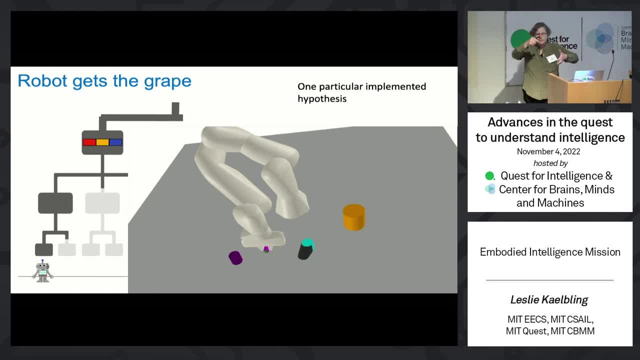 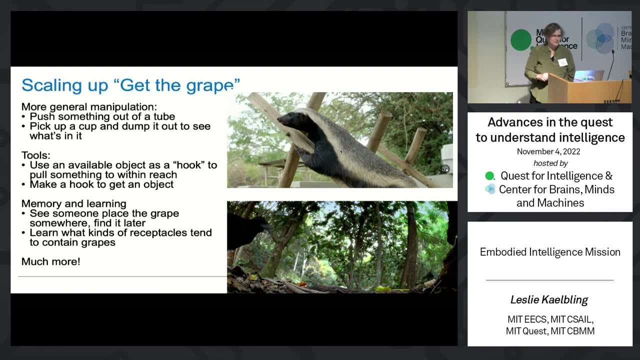 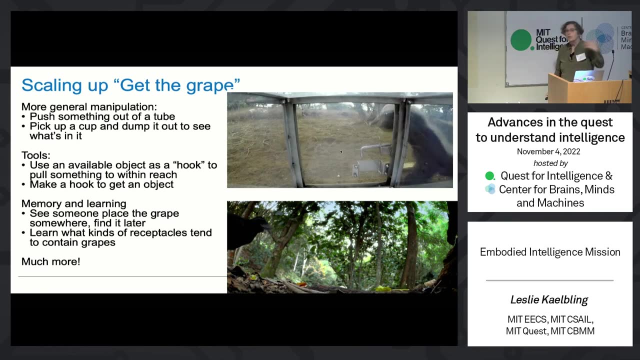 experiments in the humans and the monkeys and help refine our understanding of, for instance, how one might approach this problem. okay, so that very simple. get the grape is very simple, uh, but it it gives us just a nucleus from which we can expand a lot. so we might be interested in more general. 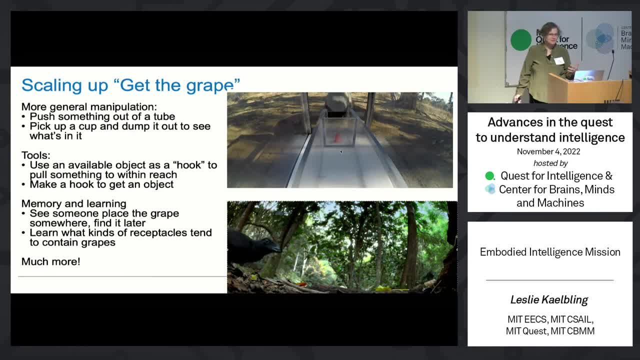 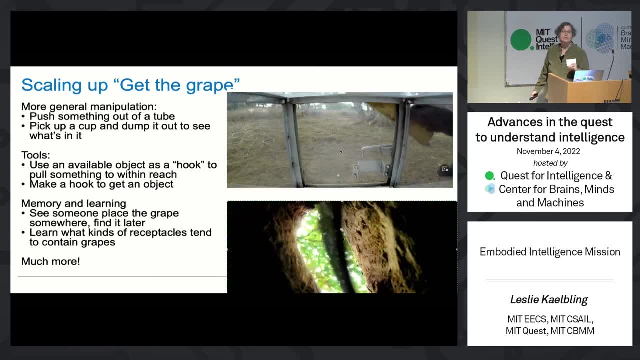 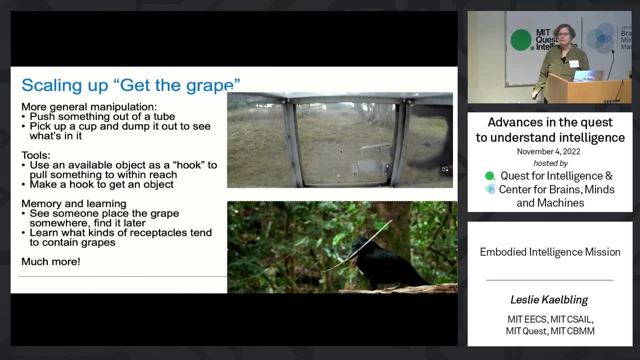 kinds of manipulation. right, so we see animals doing rich kinds of manipulation: uh, using tools, building tools, uh, studying memory and learning what happens if we show you the grape and then it away. take the scene away for a while and come back. so all of these things we can study, even 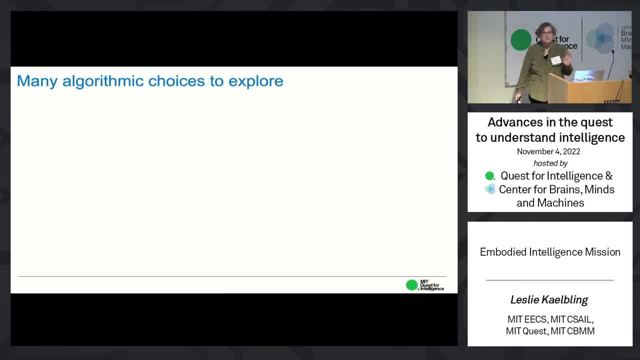 just in the context of this get the great problem and there's lots of really interesting underlying algorithmic choices. they're interesting to me as a computer scientist and they're interesting in general as questions of intelligence in cognitive and brain science. so things like the question we 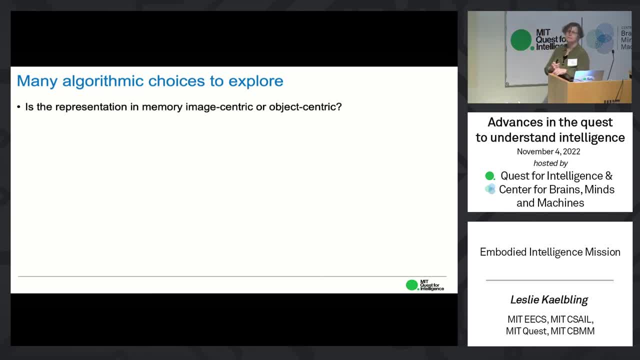 we were just asking about was: maybe is the representation in memory image centric or kind of object centric? But we can study things like: how do we organize the search for an object? Is it systematic, Is it greedy, Is it random? When should we gather more information versus when should we try? 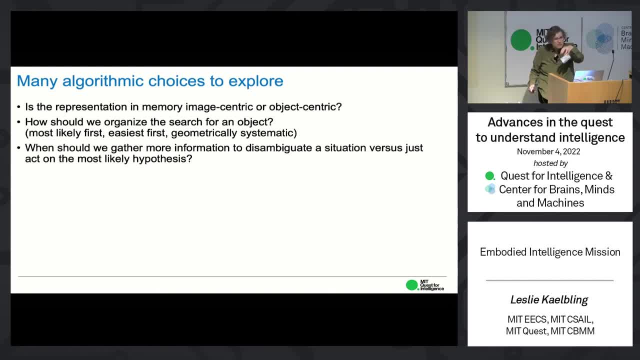 Is it worth looking around at the back of something to see what it's like before we try to move it, or should we just move optimistically? Or how frequently should we reevaluate our higher level plans and intentions? So in our computer implementation of the controller for that robot, it has a whole hierarchy. 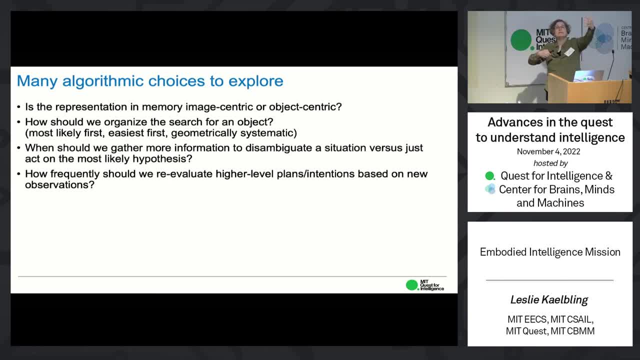 of plans And, given evidence, it might decide to just reconsider its whole strategy. But how often should it do that? for instance, How should we do data association? When we see a new object, how do we decide whether that's really a new object or actually? 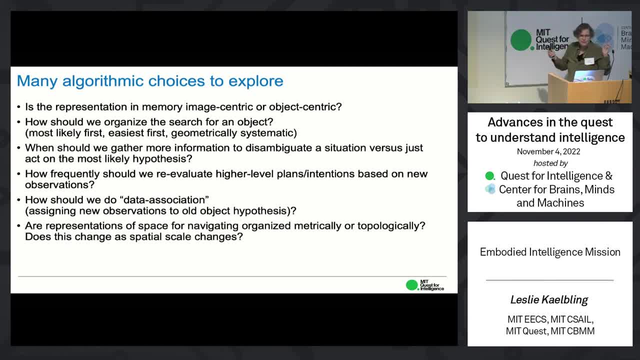 just a new view or a slightly moved version of something before. How do we organize our representations of space? How do different aspects of behavior improve with experience? So the list of questions is just enormous and it's super exciting because we're kind of poised to study these questions now in all different modalities. 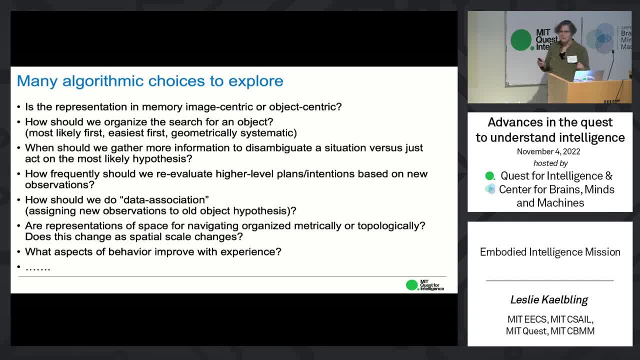 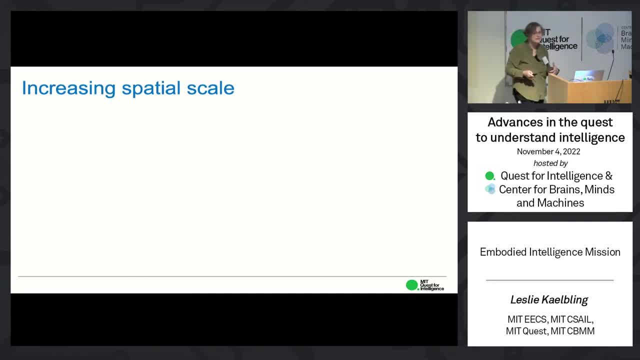 So now we can scale up even further, right? So finding the grape on a tabletop is interesting, but hardly the whole world of embodied intelligence. So one of the things that we're working on also right now in parallel is increasing the spatial scale of the problems we think about. 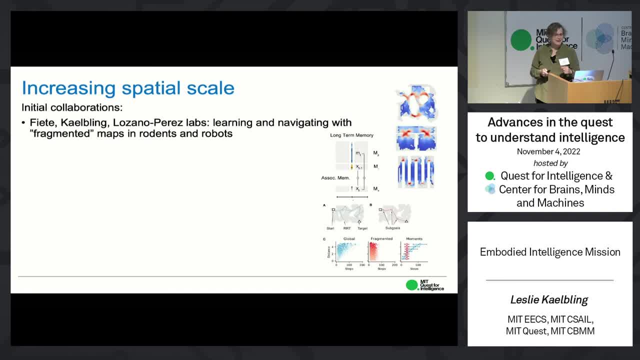 So we have an initial collaboration with Ila Feet, who's going to be speaking after me, studying navigation and how it is that that in rats and in robots we can build maps that have a kind of hierarchical structure and the degree to which that might help navigation. 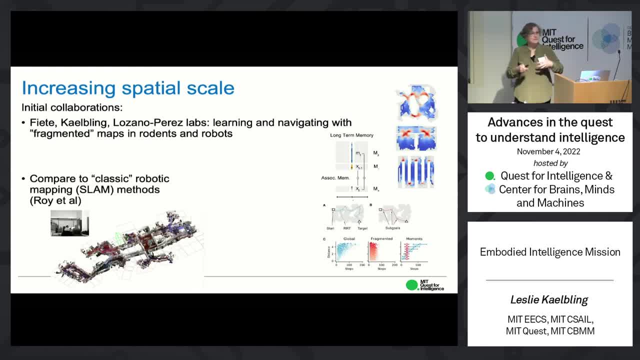 be more efficient. We can compare that to other kinds of methods that build maps that are more globally accurate, more metrically accurate, And this is work with Nick Roy, so we can extend to bigger spatial scales. We can also just extend this problem in a myriad of ways, right? 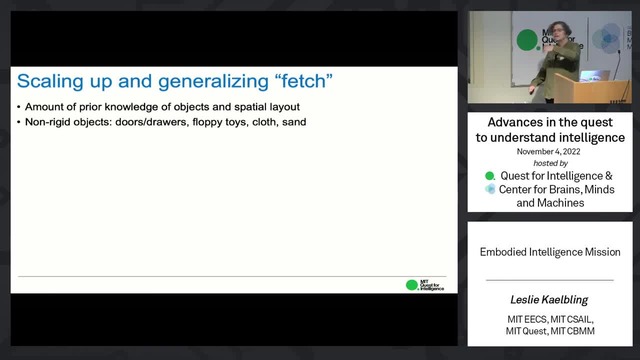 So we can study the amount of knowledge that we have have in advance. We can make the objects be non-rigid. We can really study the question of how partial information changes your strategy: increasing the spatial size, making the task complexity go from finding a grape. 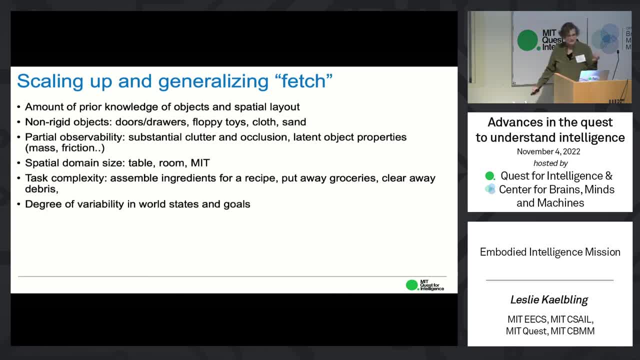 to assembling something: building IKEA furniture, putting away the groceries. We can vary the variety of situations and goals that we ask for. We can start to connect to our colleagues working on language and think about how it is that we interact with humans and other agents and how can we interact linguistically. 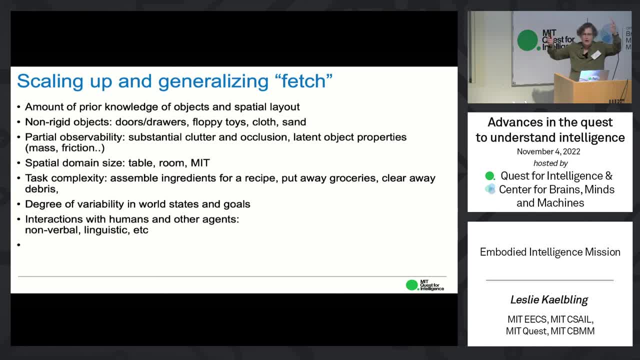 and non-linguistically in useful ways, And again, the questions just grow from here. So, fundamentally though, the important thing is that we don't want to solve each sub-problem individually. That is absolutely not what we want to do. 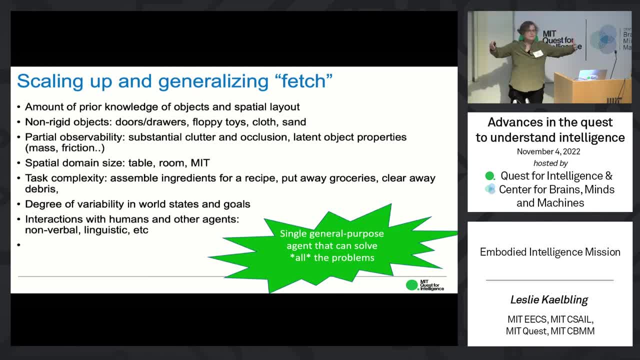 We want to understand how to build one general purpose solution to solve this whole class of problems, because we think if we could do that again we'll come back to the bet that we're making, that if we could build systems that can solve such a big class of problems. 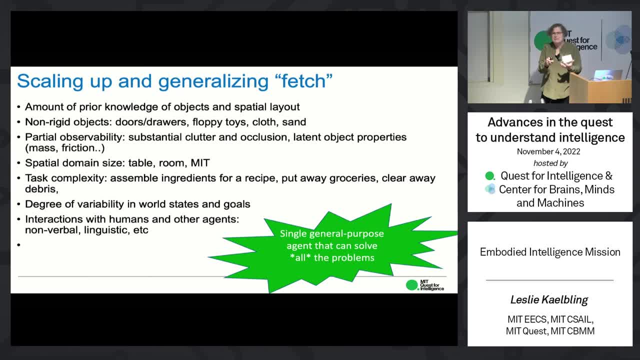 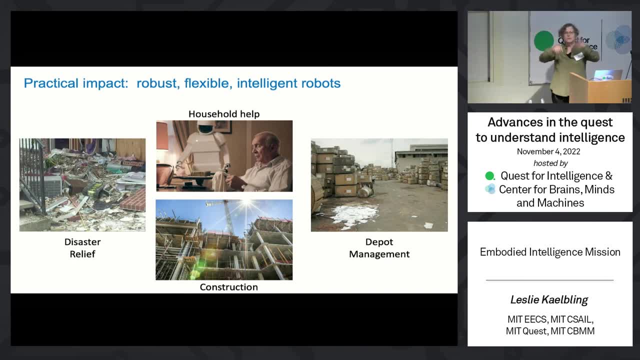 then it's most likely that they would share some underlying structure and technique with the way that humans solve those problems too. So let me just close by kind of recapping the kind of impact that we hope to have. So there's practical impact in building robot systems that 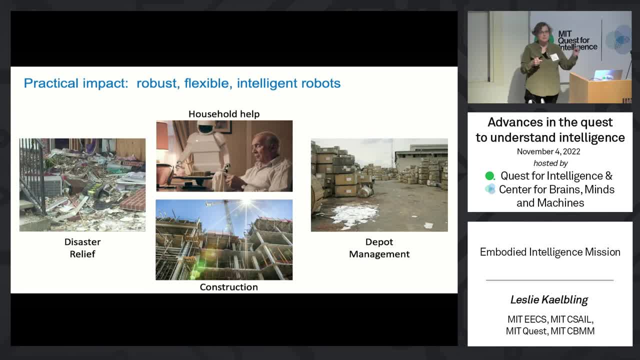 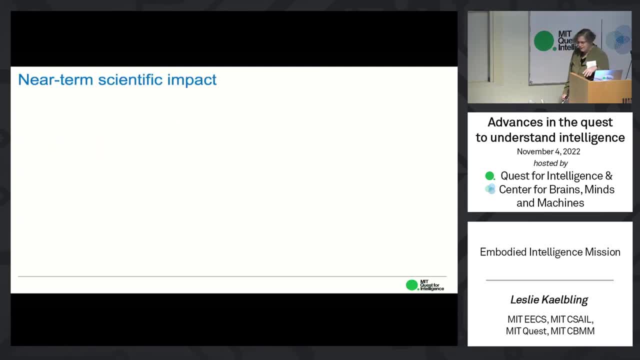 can go beyond very prescribed factory environments and out into the messy, messy world that we all live in. There's practical impact, There's scientific impact. There was the kind of grand rainbow of scientific impact that I talked before, But there's also a kind of more near-term scientific impact. 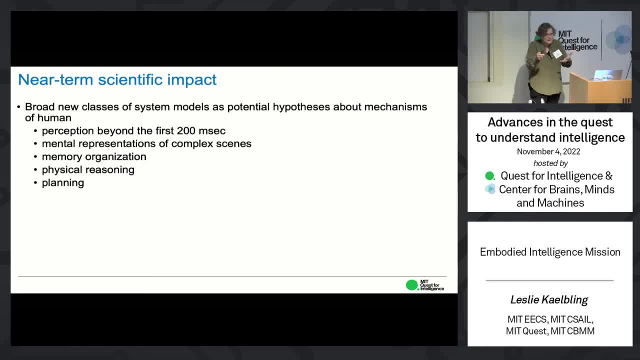 In particular. the hope here, and clearly actually the reality, is that by having this close interaction between the cognitive science, brain science, computer science, people, we can really come up with new classes of system models as potential hypotheses about mechanisms for all kinds of human cognition, including perception. 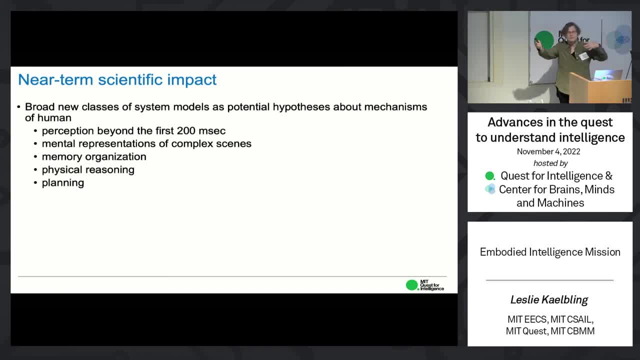 beyond the very first few layers, mental representations of physical scenes, memory organization, how you reason about the physical world, how you make plans at different levels of abstraction, and so on. And the idea is that once we have these hypotheses, then we can design more focused neural and behavioral kind. 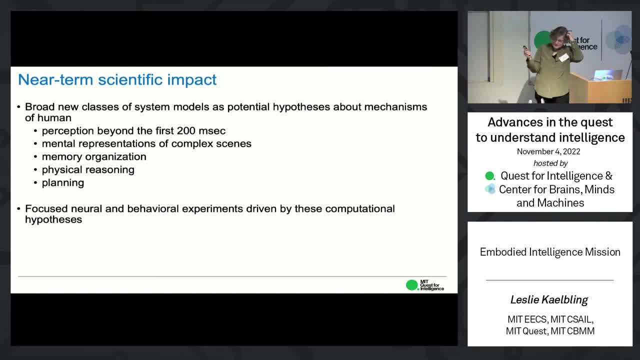 of experiments Instead of just doing an experiment and looking at the data and going, hmm, I wonder what about that. we can be really much more focused in terms of trying to figure out how to do that. We're trying to discriminate between the hypotheses. 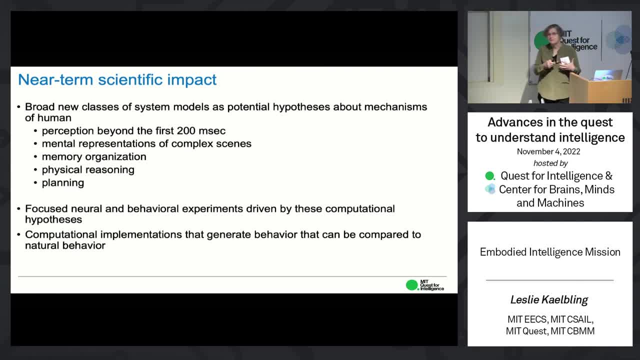 And we can maybe improve our computational implementations, And those computational implementations will demonstrate a certain kind of behavior that we can also go look for in the natural systems. So we think that this process, this sort of virtuous cycle of going around between constraints that we get from experiments in nature, 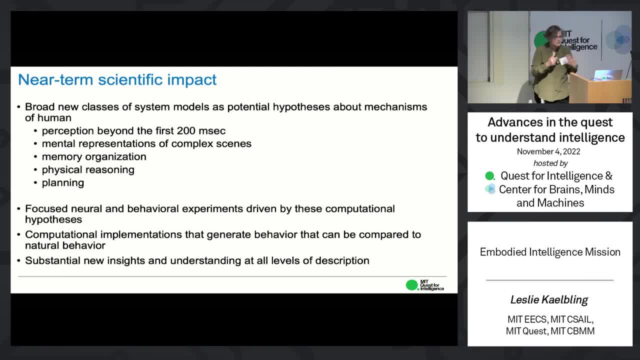 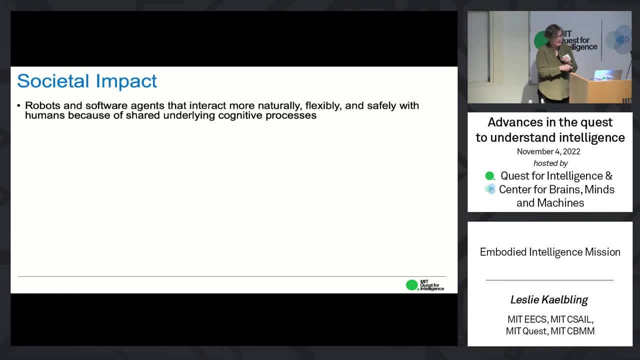 constraints we get from implementation. new hypotheses and so on will give us really new insights. in all of these different realms We also hope to have a real impact on society. One important type is the idea that if we build robots and software agents that have in their underlying structure 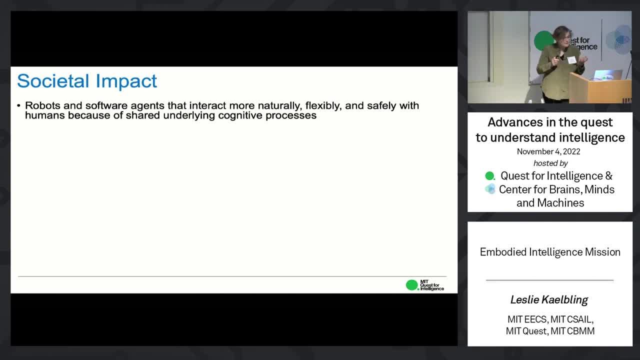 and processes a similarity to humans, that these systems might be easier and more natural for humans to interact with. We also think that if we build these systems that have some amount of engineered structure in them, it will be easier actually to understand and verify them. 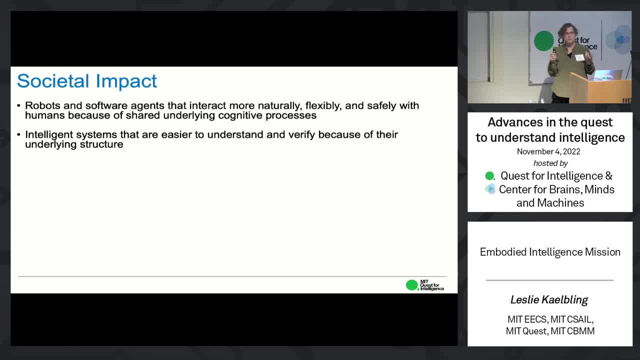 to trust them, to believe that we understand what they're going to do in more complicated situations, Because we can actually kind of look inside the implementation and see what's going on, as was true with our robot that was looking for the grape, The robotics. people like to talk about tasks. 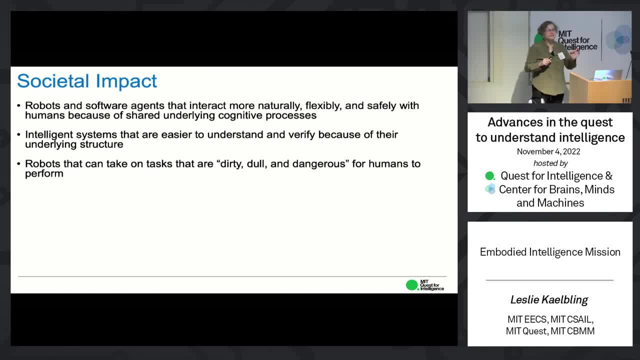 that are dirty, dull and dangerous. So that's a kind of a watchword for a category of jobs that humans find unpleasant or difficult and that maybe we can make robots take over some amount of that work, subject to a bunch of things.